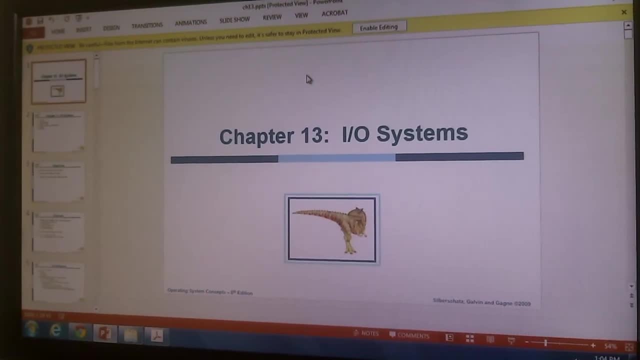 And I'll give you the tips and hints about the questions. And the questions will be. first of all, there's no programming questions, no coding. That's good for you, right? I know it's going to take a long time to write. you know a couple of lines. And the other thing maybe multiple choices and no definitions. There will be no definitions at all, zero. 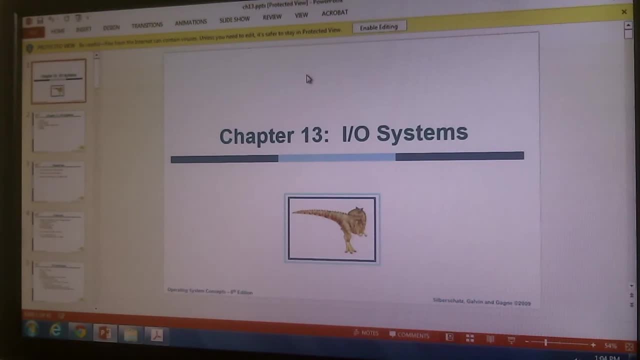 And most of the questions will be- I'll give you a problem, you'll give me a solution for that- And some maybe true-false questions too you will have. It's going to be pretty easy. If you understand the subject, if you know the logic behind the stuff, then you'll be easily able to, you know, answer the questions. 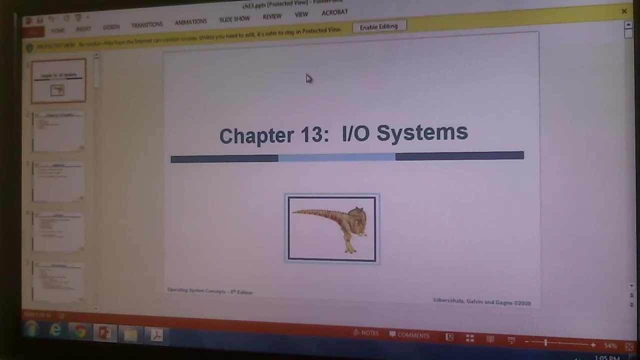 I may give you a graphics and talk about it. what you think? What do you see here? What do you think what's happening here? You know, you remember that CPU course with the processes, Something like that probably. And yeah, we will talk about the other type of questions later along these slides, at the end of this class today. 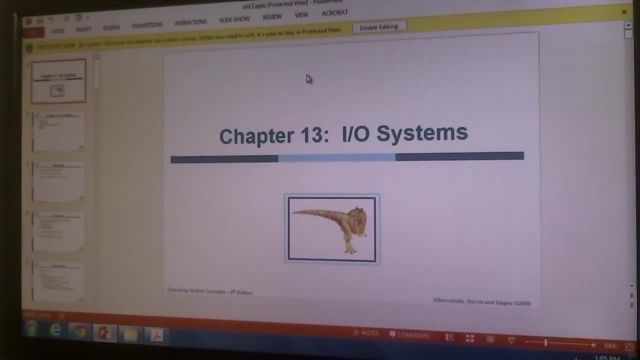 And the good news. you know many people are telling me that. you know it's a waste of paper. you know just if you don't use a laptop Or you know smart devices, you know we cannot really copy, print out lots and lots of stuff. It's not really good for us. 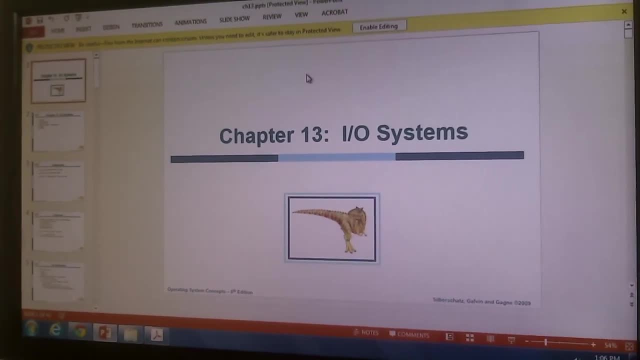 I agree for two reasons, not for the trees, but for the. at the beginning of the semester I was saying that all the examinations, if there's any tests, and the final examination will be open book And you'll be able to use your laptop, whatever, etc. I said that at the beginning. So maybe, probably and most likely, yeah, you can use the laptop. 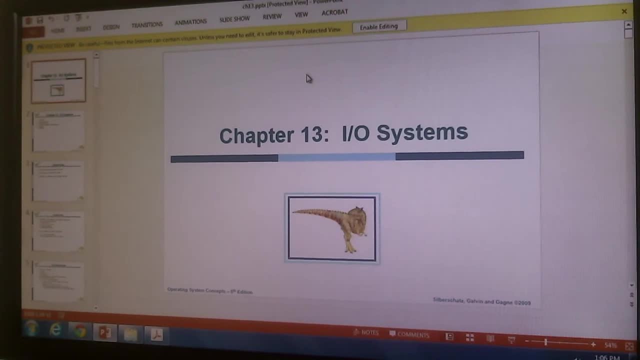 For the test. Yes, for the test. That was the announcement at the beginning of the class semester, but later on I changed my mind. I said you can't use it. But you know, whatever, now you can use it, It's alright, Okay. 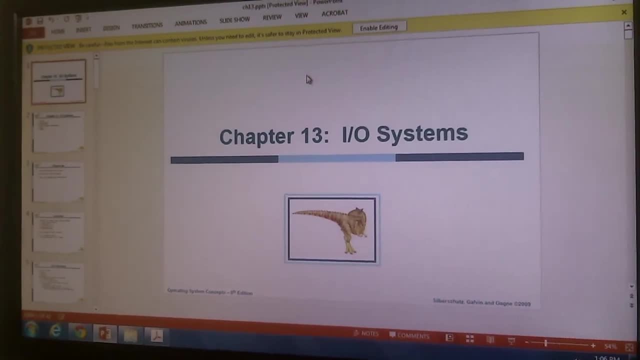 You can use a laptop, but you cannot use a smartphone. Okay, Wow, You can use a laptop. You can use a laptop because the textbook is more than 600 pages And I know you're not going to print anything from the textbook, but probably you want to print out the slides. 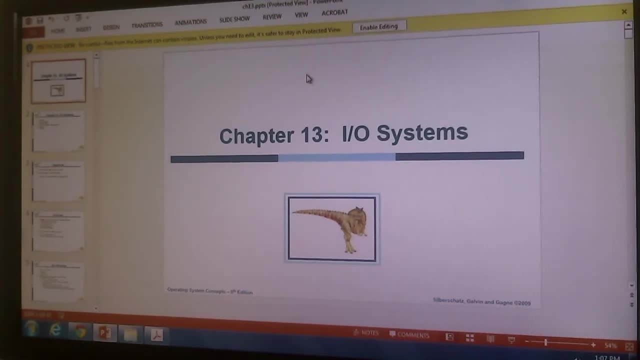 But even the slides. it's a lot. So printing out those stuff is not a really good idea. But in general in regular, you know, for all the other classes you don't need to print out anything. You're not allowed to print out anything. 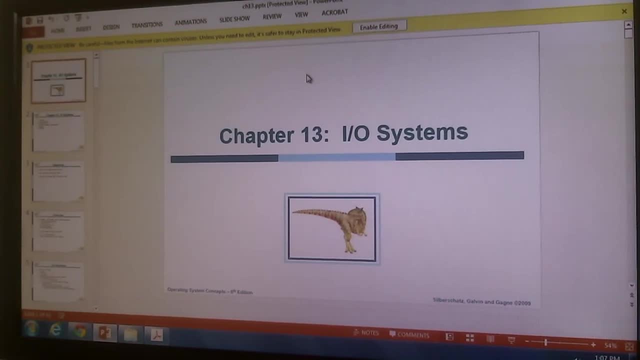 You're not allowed to get a cheat sheet or anything You're supposed to know in here. Right, You know you can't use a laptop, you can't use a paper, anything. But in my classes- most of the classes like 99.9, I allow students to use any kind of resources they have, because I don't really want you to memorize stuff. 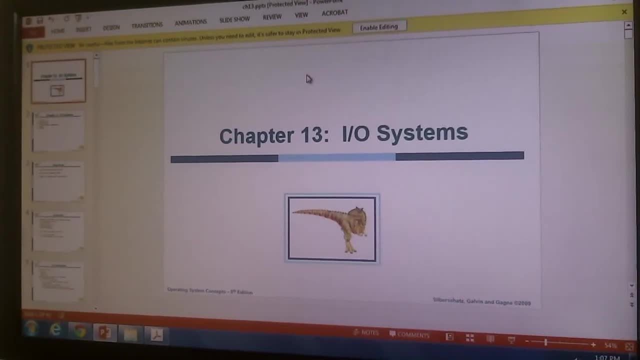 I want you to know the stuff, Alright, But sometimes you have to memorize. specifically, if it comes to the programming, You have to memorize stuff, Right? Anyways, today's chapter. as I said at the end of today's chapter discussions, I'll give you a review. 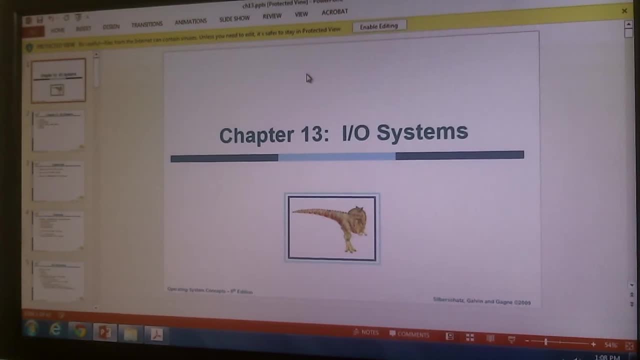 So tomorrow there is no review. I mean, you don't have to come Tomorrow and Thursday at 1 pm is sharp The exam starts and you will have three hours to finish that, Let's start. Any questions? No, Okay, 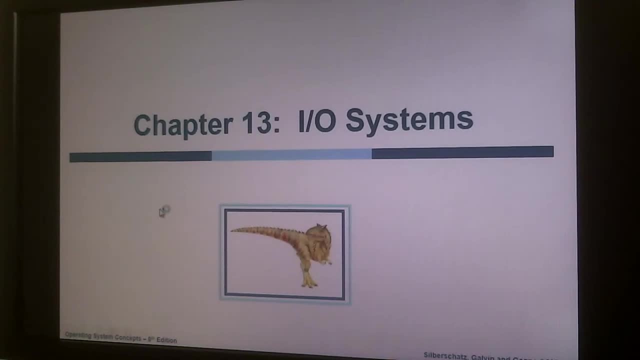 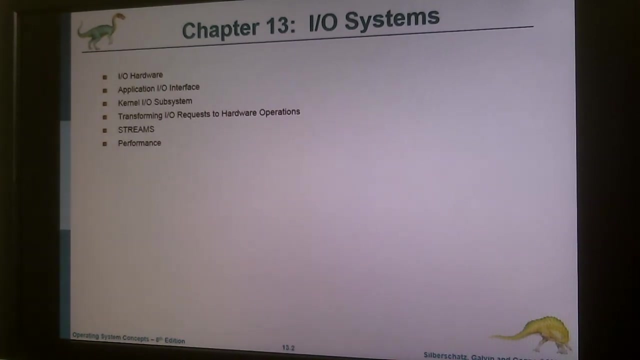 Today's chapter is IO systems. We're going to talk about IO systems. It's one of the responsibilities of the operating systems. Alright, And what do we do with IO systems? First of all, it's more like computer architecture here. 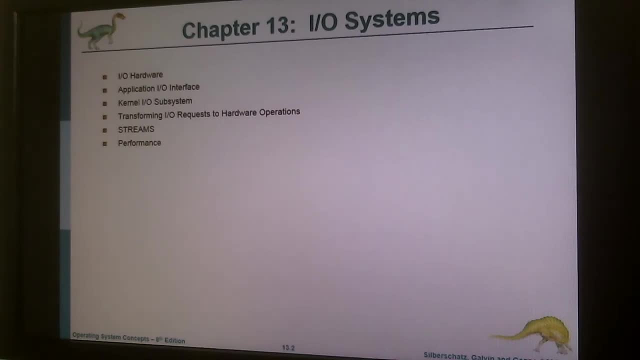 You're not going to talk about any algorithms or anything, But we will talk about the inner workings. Again, this Chapters in the textbook is always talking about general stuff. We're talking about a generic operating system, Alright. And at the end of each chapter we have some examples about Windows XP, Windows NT, Unix, Linux, Solaris, etc. 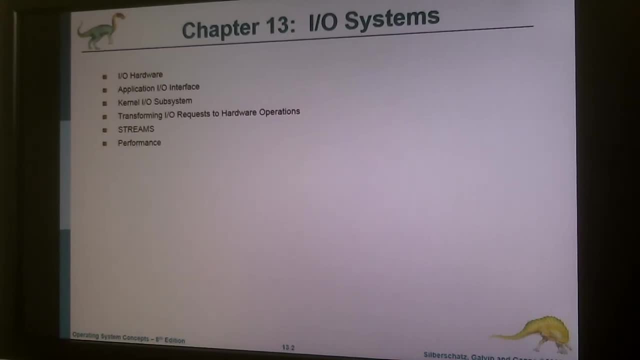 What is an IO system? Why do we need any kind of IO system management module or application in our operating system? Why is it a part of a kernel? That is the main question. That is the first question You might have. 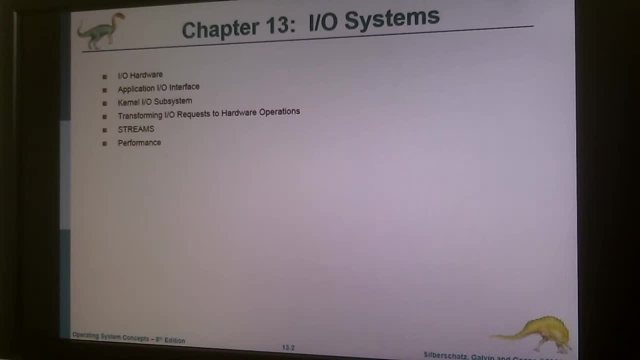 Here. what is a computer? It's a bunch of hardware, right? Yes, You have your CPU, you have memory, you have other electronics in it. You have also hard drives, CD-ROM, etc. Without any operating system or without any application. it's nothing. 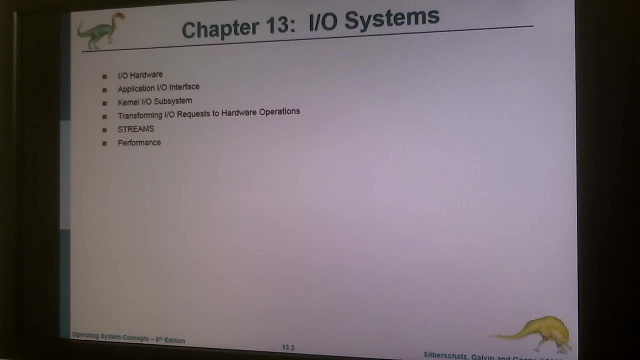 It's just a tool, but you have to make it work. For that reason, we need an operating system right, But so far we were talking about the processes right And we were talking about CPU and memory management. It was just okay to handle lots of jobs. 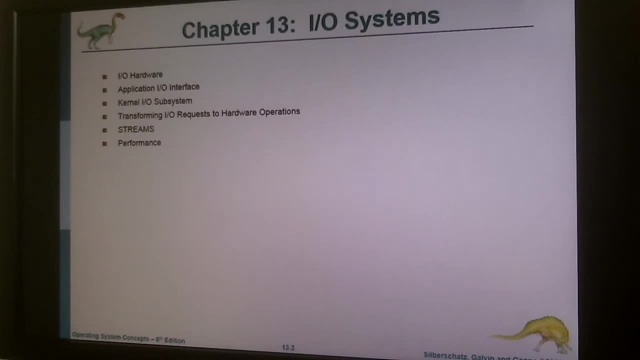 You know, you wrote an application in Java, for example. Oh wait, hold on one second, I'll give you a chance. What is it today? 11, right, If you have a program, if you have a user application, in any language, 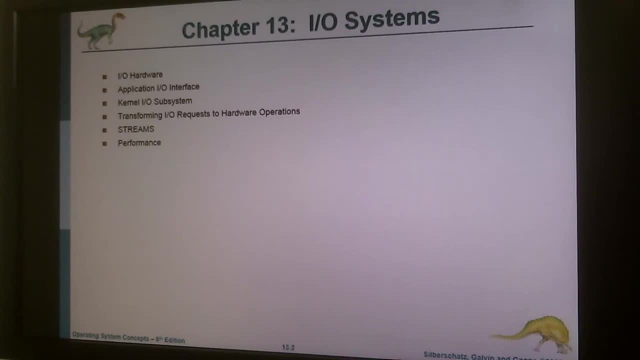 all you have to do is transfer that application into your hard drive, install it and make it run right. You just need the CPU and the memory. But the problem is here: How are you going to reach to your hard drive at first place? 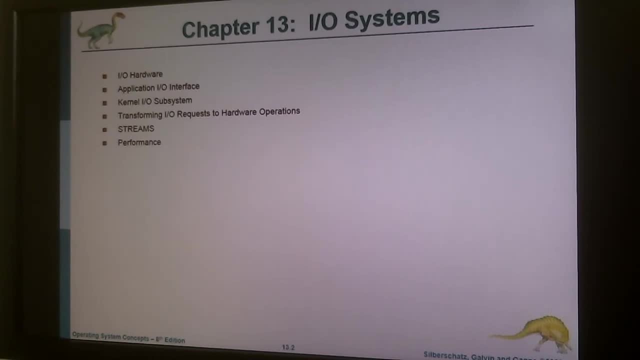 At the very beginning. how can you install your operating system on the hard drive? That is the first question. That is the first problem, right, And when you fix that problem later on you will be able to install your applications and run them with no problem. 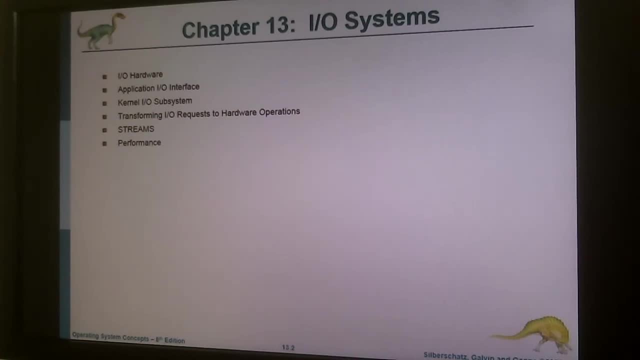 because we already know CPU and memory are manageable by the operating system with no problem at all. There's a lot of algorithms, system calls and everything manages the CPU and the memory. already right. But we didn't know anything about the hardware. We were hard drive. 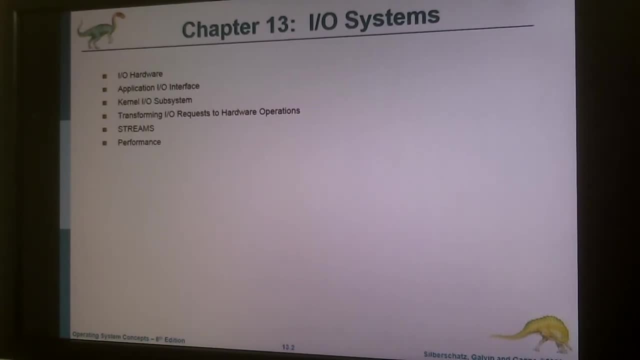 We were just saying that you know what you need. You need a file name to open. Once you open that file, you can read, write whatever you know, delete, rename the file, etc. You could do those stuff. 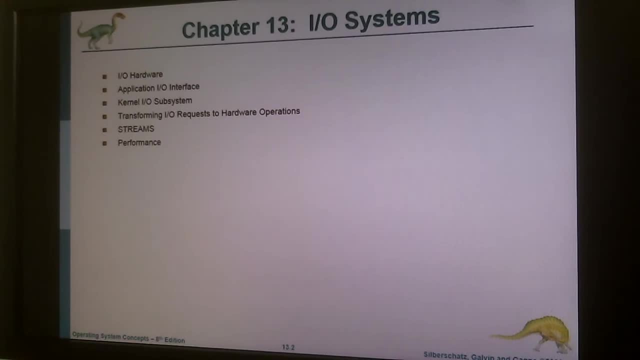 But we didn't say how you can do it. You know, as a programmer, as a developer, you don't have to know the inner workings, but as a computer scientist, you need to know them. By the way, if you want to know more about hardware, 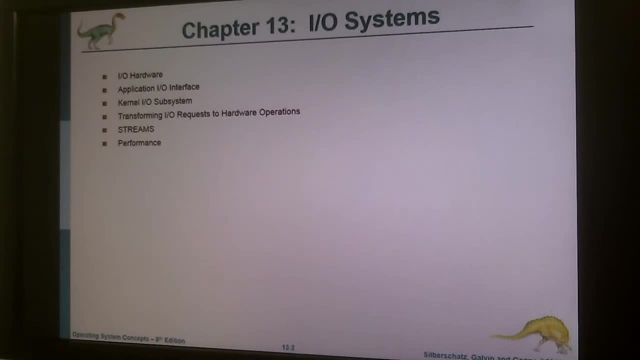 and you want to be able to build your computer from scratch. you want to buy motherboards, CPU, memory, hard drive, a case, a monitor and put them all together, install an operating system, make it work. If you want to be able to do that, 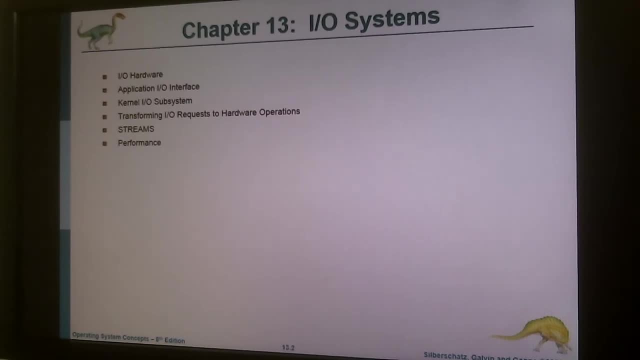 you need some sort of tutorial, most likely an A-plus book, a CompTIA A-plus book. You can learn more computer architecture stuff, Hardware stuff from that book. Most of the jobs as a computer technician in the market right now they require A-plus certification from CompTIA. 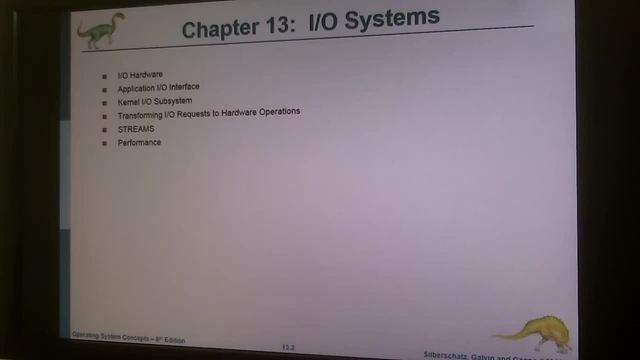 You just study that book, pass that exam, get some hands-on experience. It takes only two, three months and then you are a computer tech. You don't need a university degree for that, You don't even need a bachelor's degree. 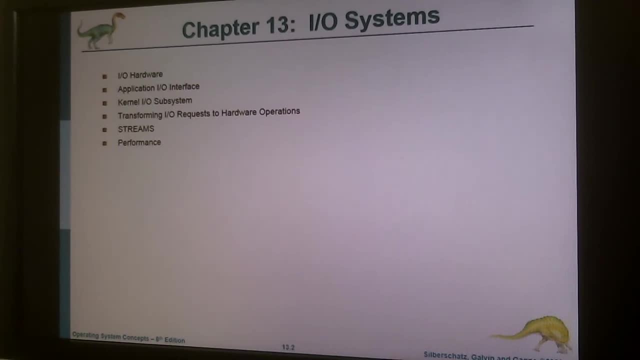 But most of you here are graduate students, right? But if you just need to know about those stuff, you can get that. That's a resource I'm just letting you know. And also, when it comes to the certifications, when you're applying for jobs. 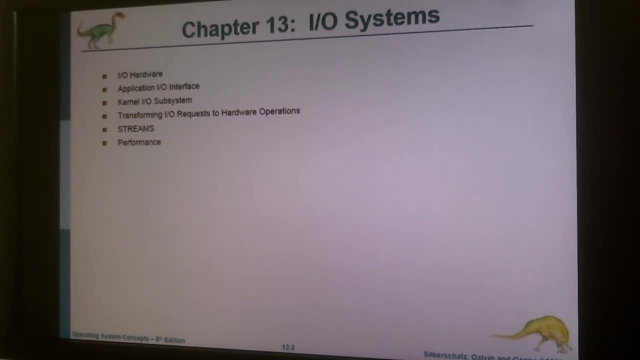 some of them are asking for Microsoft certifications like Microsoft Certified Professional, Certified System Engineer. Some of them are asking for Cisco certifications like Cisco Certified Network Accession And others. What was the one you're after? CCNP, CCNP, Network Professional. 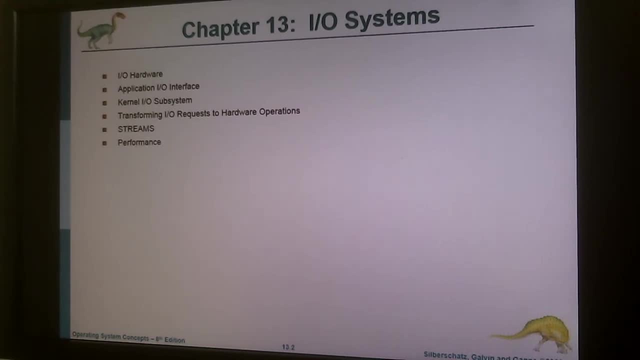 Okay, So one or more depends on the certification. You're going to take one or more examinations. If you pass them you will get the certification. But there are two types of certifications in general: Paper certifications and real certifications. The paper one you go ahead and search on the internet. 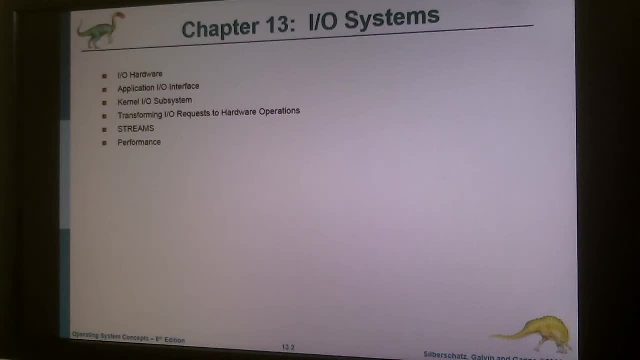 Find those, Find those questions and answers from previous examinations and then memorize them and get the examination. You will pass straight with 80, but you will know nothing. That is called paper certification. The other one: you got real hands-on experience. 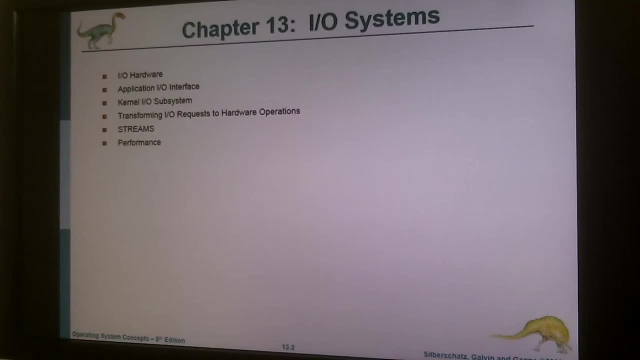 You can get those from the private courses, or you can just go ahead and buy some stuff from Craigslist or some cheap stuff or used stuff like Cisco routers, switches etc. Or what you're using Simulator, Cisco Simulator- What is that called? 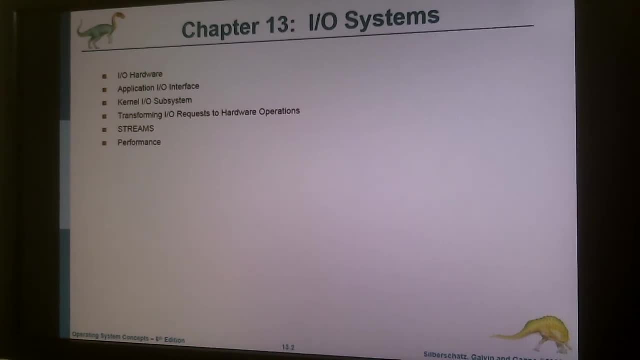 Logos. It starts with a G. I forgot that too, But you know it starts with a G. What was that GNU? Anybody has any idea about that? simulator for Cisco examinations, certification exams, A simulator which simulates routers, switches. 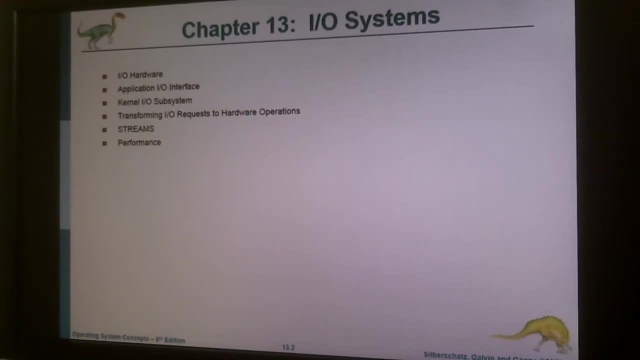 and other stuff, firewalls that you can log in and it's a real-world, you know, experience-like environment. Okay, it starts with a G. Anyways, if you're interested, you can search on the net. What is the best simulator for Cisco certification examination? 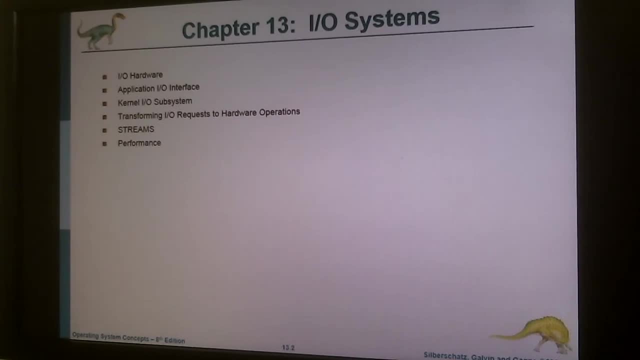 So you can figure it out. Anyways, you know those companies are asking for those Certifications. If you have a BS and a couple of certs, one or more certifications, you will just be one step ahead from the other candidates and you can get the job easily anyways. 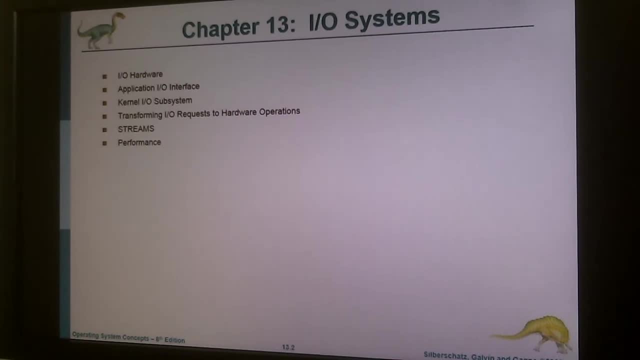 But certifications are not mandatory. It helps you to open the doors, Anyways. so in the IO systems, IO subsystem is a part of the kernel, It's a part of the operating system, All right, And it handles all the IO inputs and outputs. 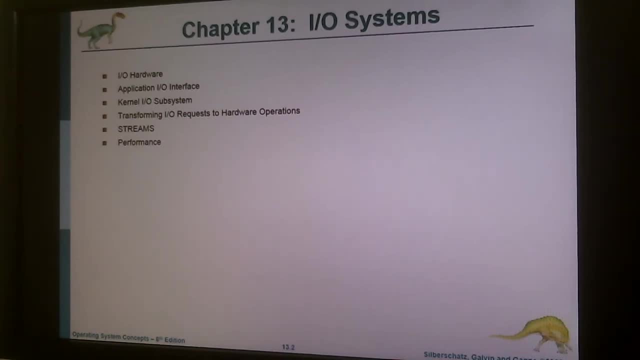 But it does it in you know, a couple of different ways. We will see what kind of approaches available for us and in modern operating systems which ones are used mostly. All right, The objective of the chapter is explore the structure of an operating system's IO subsystem, blah, blah, blah. 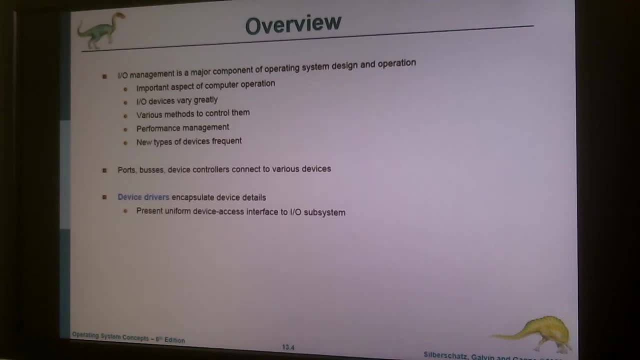 Okay, With the CPU and the memory you have CPU scheduling, memory management, paging, virtual memory management, et cetera. right With the IO system, these stuff are working super fast, Relatively, of course. You know we're talking about speed, about milliseconds. 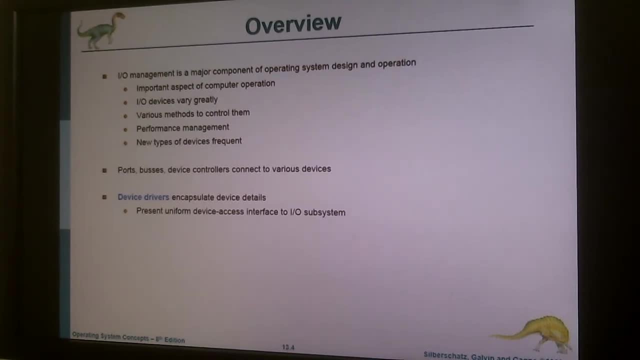 around milliseconds- one to ten milliseconds. But when it comes to the IO systems, the story will change a little, because CPU and the memory are fast stuff. right, They're super fast. For example, three gigahertz CPU and the memory speed is. 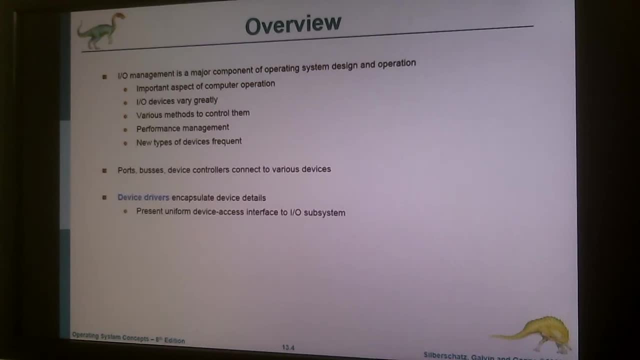 how many megahertz. right now I don't know What is the latest one. If you just Google one, go to Amazoncom and type DRAM, you will see that 110,000 megahertz, one gigahertz to two gigahertz. 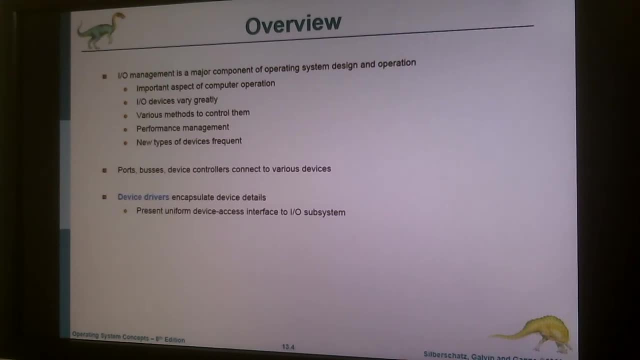 It changed. Anyways, it's all around gigahertz, right, But it's not the same for hard drives, CD ROMs and other IO systems, And most likely as a user when we say IO devices. 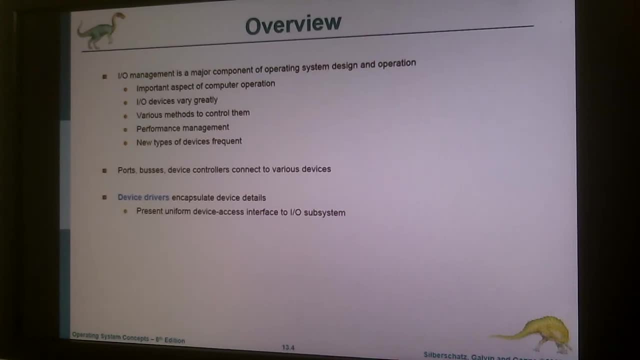 we always think about a couple of stuff like hard drives, USB drives, USB flash memory sticks, right And printers, cams, video cams like this one here- keyboards, memory, What else it could be, And this is like you know, everyday user could see or use. 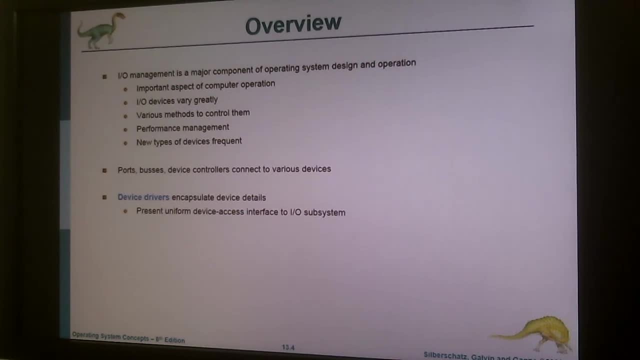 But there are some other types too. It's not only limited with the things you see on the Best Buy. There are a lot of different types, For example, a retinal scanner, a finger scanner, fingerprint scanner. It's kind of unusual, but you can still see it on Best Buy, right. 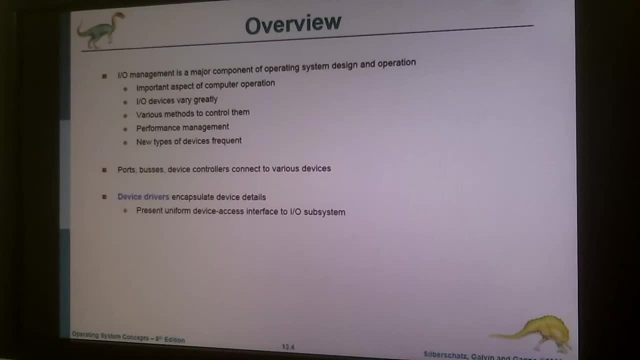 What else? What kind of IO device you can think of which is rare? Give me an example: Like the printer that we have, LPD ports, LP. what LPD ports? Like the long ports, the dot matrix printer? 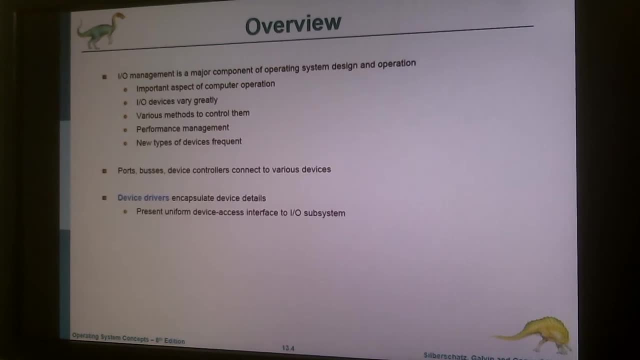 Dot matrix. Wow, How old are you? I'm surprised somebody knows about that. It's been years ago. Are they still in the market? Not really, But some actually. yeah, some of them should be around because It hard copies multiple papers, right. 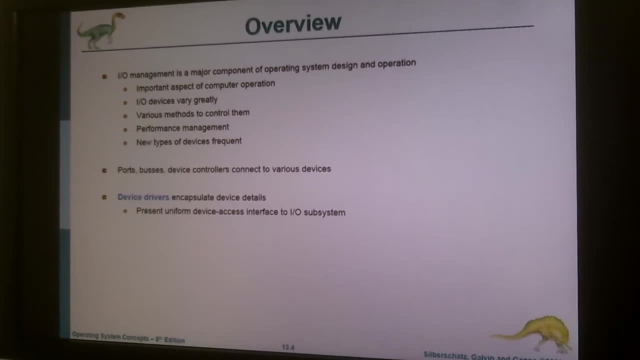 You know it's required for some governmental stuff, so they might be in use. still I don't know What else. Let's say you put a computer on a Mars rover- Again, SpaceX stuff. Come on, You have the Mars rover. 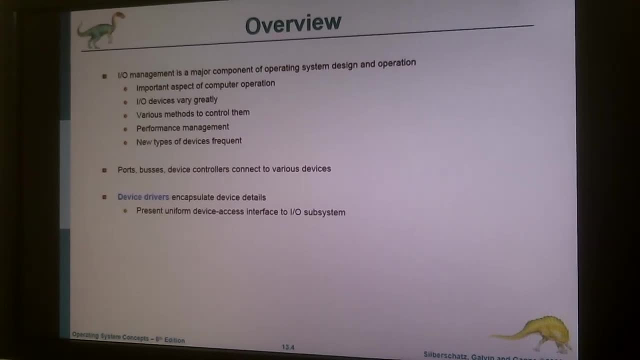 Oh, forget about that. Mars rover. Come on, You have a car, a modern car. You just bought it 2015.. You have lots of stuff right. You have a large screen, GPS, It shows the maps, It shows rear camera things. you know. 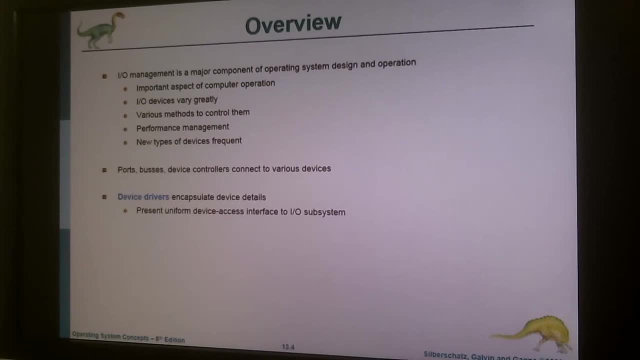 Some of them even have ultrasound scanners to you know. warn you if you're too close to the car in front of you, If there's somebody at the back while you're going backwards, it just warns you. What kind of sensors we are talking about. 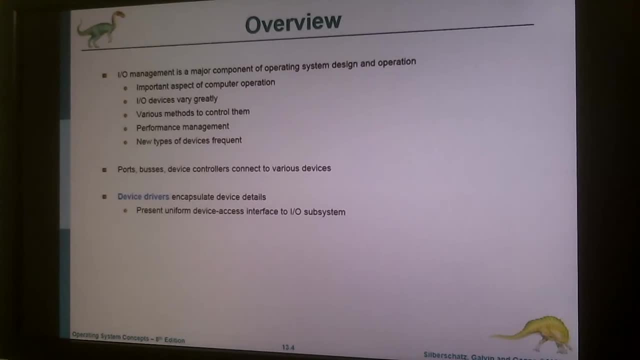 Let's say motion sensors, right? And do you think there's a computer inside the car somewhere? Yes, Yes, there is right. And they're even talking about hacking into those computers and, you know, taking over the control of the car. 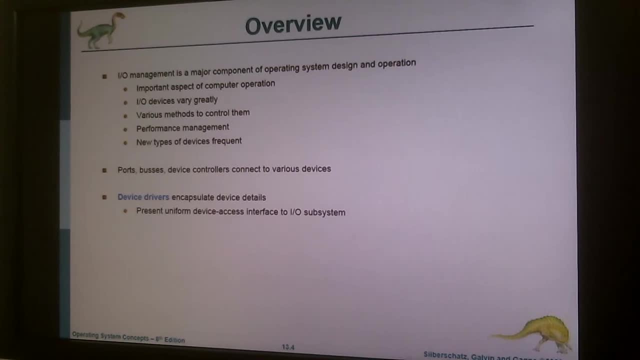 without you knowing. You know you're sitting in your home and your car is parked and they hack into it and then they just turn it on and then they use the you know, like in the James Bond movies. Yeah, They can just take the car. 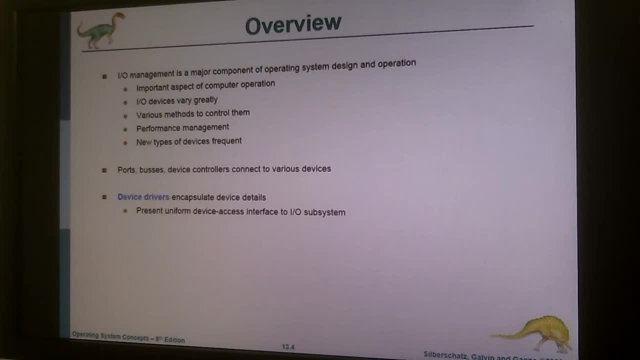 They can even drive the car driverlessly- right, They can do that. Tesla had that problem. They fixed it already, for example. So what kind of eye device we're talking about? The sensor, the motion sensors, It's a real different kind, right? 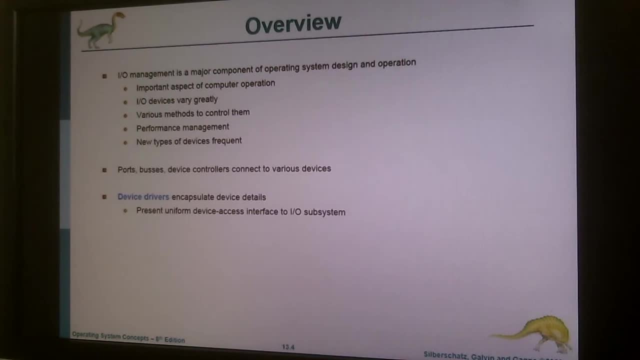 I mean there's a computer inside it. For example, Tesla works on Ubuntu. The operating system in that computer is Ubuntu. I don't know about the other cars, but it's an embedded system. right, They have an operating system too. 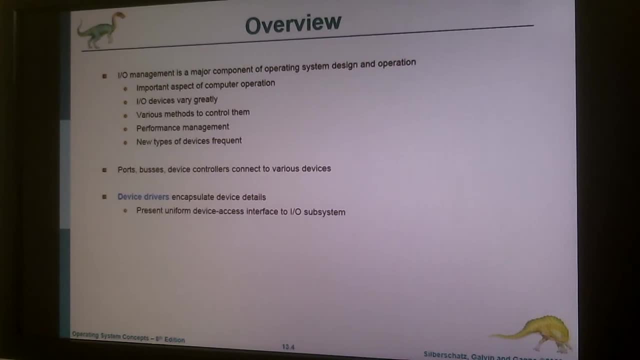 And they have sensors and other stuff attached to that computer. These are also eye devices. So our topic today: we're going to have to teach our operating system to manage those sensors, manage those printers, keyboard, mouse and other peripherals, you know, attached devices. 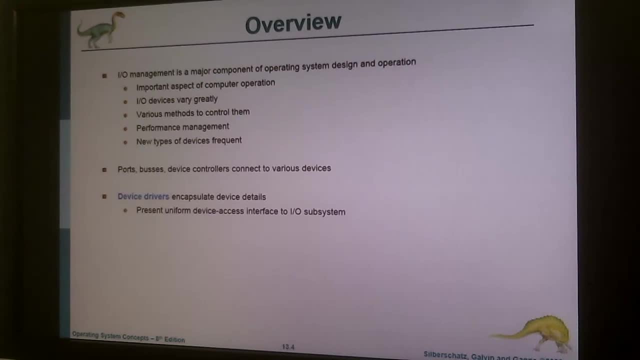 Anybody know? Anybody heard about Plug and Play Windows? Plug and Play, I heard about it. Yeah, What do you think it is? Do you know how it works? It's supposed to be able to connect to a wireless. correct. 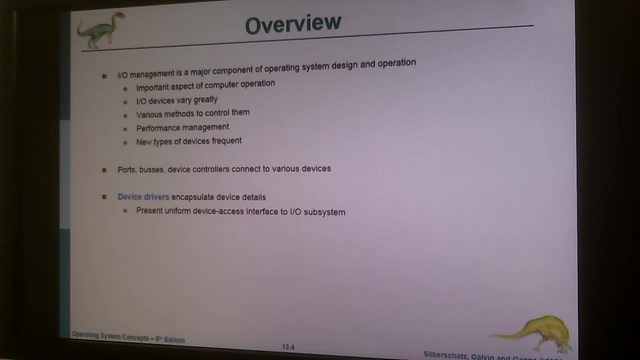 Isn't that what it's supposed to be about? No, Plug and Play is like Android and Flash Drive. also, It's like You said. there are some Android devices like Plug and Play, like you can control your phone through the smart TV. 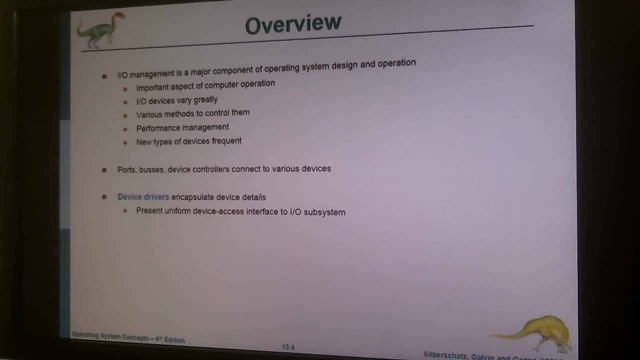 like it has the Android device. Well, no, They actually introduced that Plug and Play thing with Windows 95 years ago. What does it mean? It means: whatever device you plug into your computer, it will just run with no problem. Plug it and start playing with it. 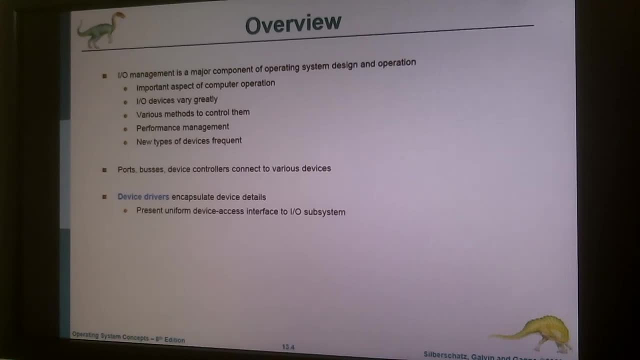 That was the idea behind it And how it works. it's a topic actually today. Again, it's about IOs. All right, If you remember the motherboard picture, I don't want to bring it up again, but there's a CPU memory and other stuff and there's also north and south controllers, right? 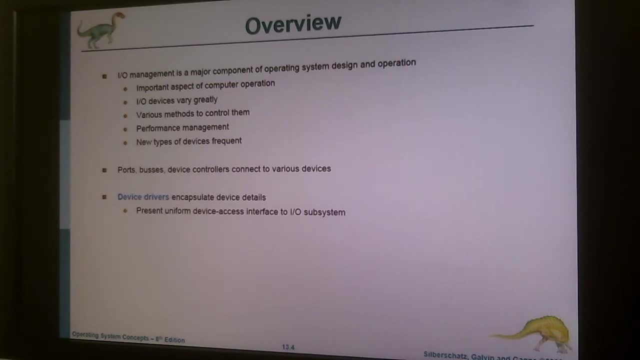 These are IO controllers And always about, when you're thinking about computer stuff, you should always think about data, code and addresses, All right, And those data and the other stuff are traveling inside the computer, through the motherboard, through the wires, those copper wires. 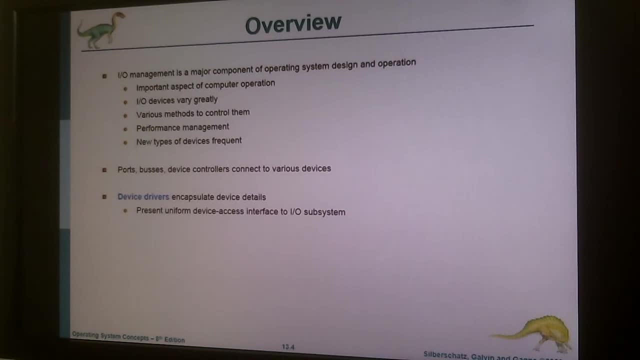 For example, if you move a data from the main memory- physical memory- to the CPU, it goes through the copper wires and then reaches to the CPU at the end. Okay, And there's a specific bunch of lines. It's called bus, which carries black code data. 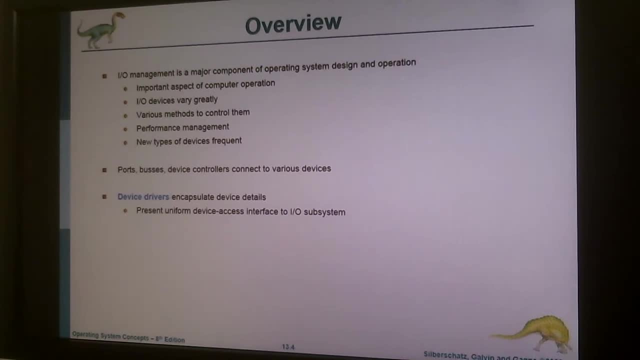 All right. And for IO devices, for example, for memory, you have a data bus And to control some stuff you have control bus, You have IO bus, input-output bus, which means those lines are specifically designed, They're assigned to those specific signals. 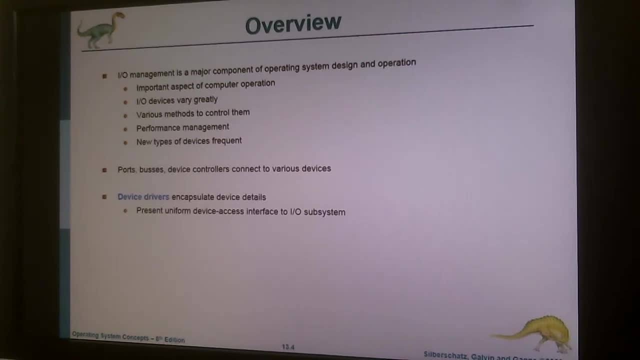 For example, IO signals are carried over the IO bus but they're not going through the memory lines, right? They're disconnected, They're not really related. So for those IO devices we have the IO bus and whatever device you plug into your computer. 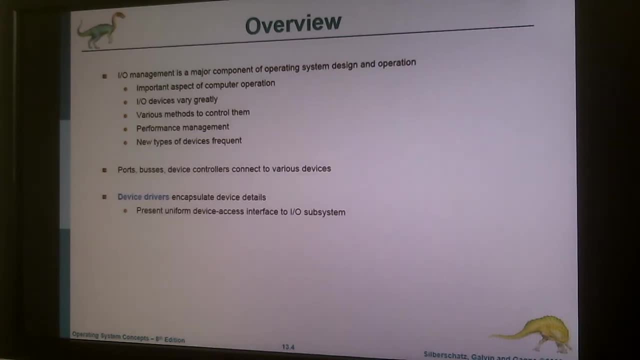 it will be communicating with the operating system through those lines, All right, And we use device drivers in the operating system. What's the reason for that? Let's say I'm trying to get data from this webcam into my computer. Is it recording? by the way? 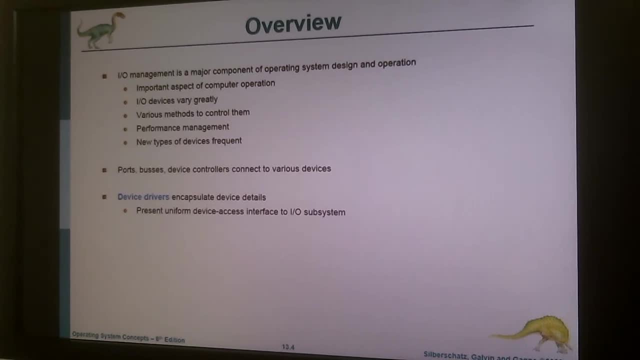 Yes, And obviously there's a- you know- optical sensor in it, All right, And that thing converts light into digital signals And that raw data goes into the computer right Through what, The USB port. But how it's possible to read that raw data? 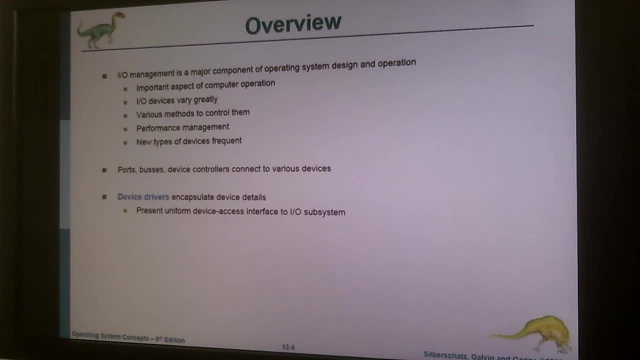 and then show it on the display like a regular picture. So this is a device, This is an IO device, input-output device. right, This is actually just an input device. It doesn't output anything. It has a microphone, It has the camera on it. 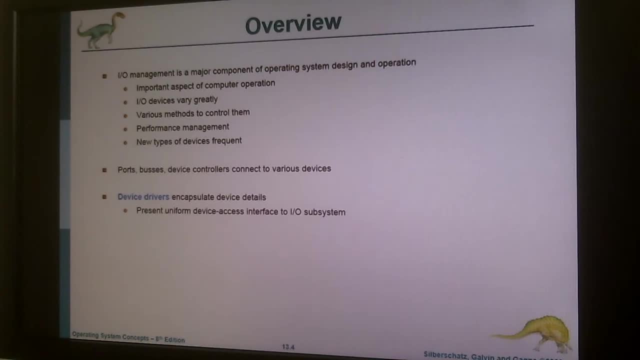 It just takes data and then pushes it into the computer. right, But the computer doesn't understand what kind of data comes in. The only way for it to understand it, you have to tell the operating system. hey, incoming bytes should be interpreted. 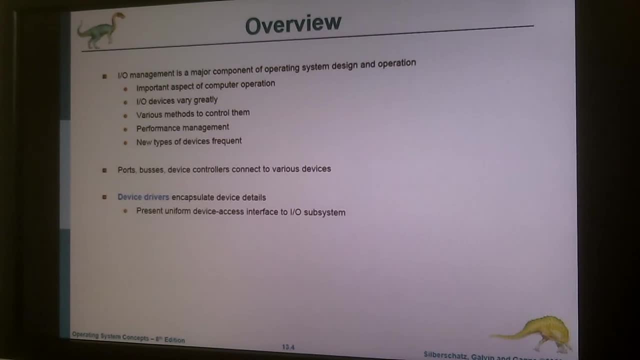 as a picture. The first bit, for example, is the black and white or color picture value. The second bit is the depth of the pixels, et cetera, et cetera. So you have to teach the language of the signal. 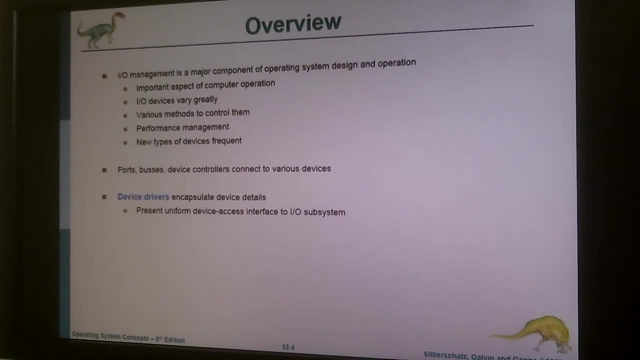 to the operating system so that it can handle it right. It can save it as a file, It can show it on the display, et cetera. So we have zillions of devices, millions of devices on the market, right? 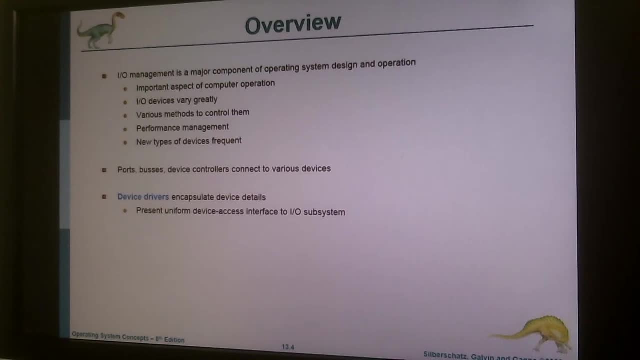 For example, for this camera. it works on the USB, It has whatever megapixels, And the other one is just black and white. It connects to the computer via serial port And you have this fingerprint scanner IO device which works with the HDMI port, for example. let's say: 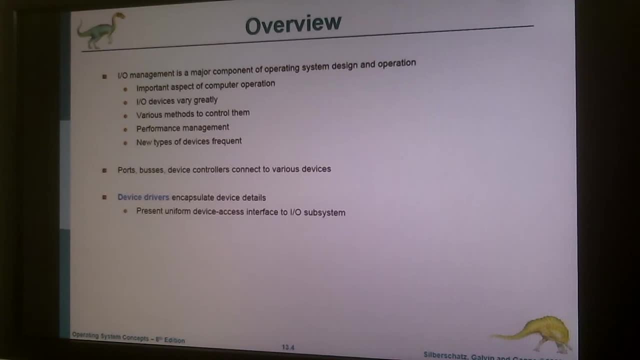 You have other stuff which needs a pilot port on the computer, So you have unlimited number of devices and one single operating system. let's say, if you're talking about Windows, How can you add those codes to interpret data for each IO device in your operating system? 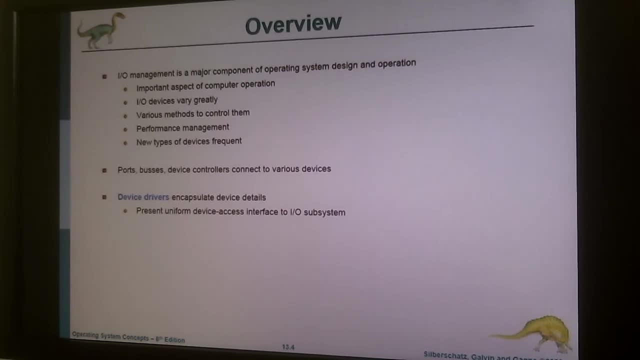 so that it will just work with those IO devices with no problem? How is it possible to write code for each device in the operating system? So what happens if there's a new IO device in the market? Do you have to recompile the whole operating system? 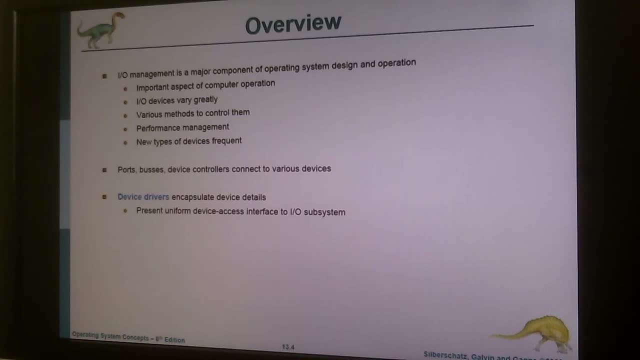 Insert the code and recompile it. What happens if you don't have enough space for all those IO device codes? It's really nonsense to add all the codes for IO devices for each IO device into the operating system. It doesn't make much sense. 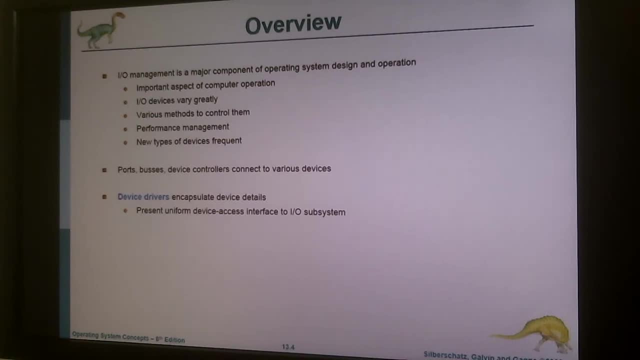 because there's unlimited number of IO devices in the market. So the solution to that is using something called device drivers. So the operating system will have an interface, an abstract interface, just like in Java. In Java you have the interface, But the inner workings. 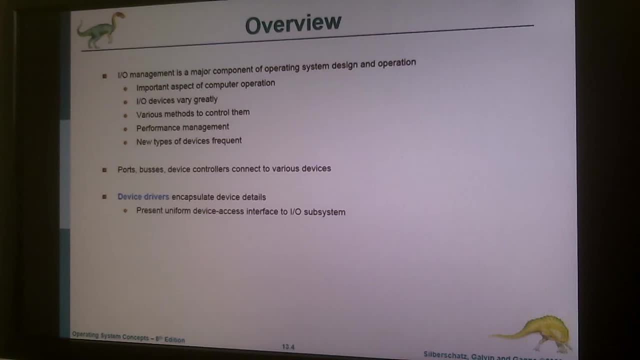 the real code or the methods in the interface depends. You can change it, you can rewrite it, you can recompile it, or you can just give completely different methods code for the same interface. You can do that, Actually, that is the reason we are having those interface files. 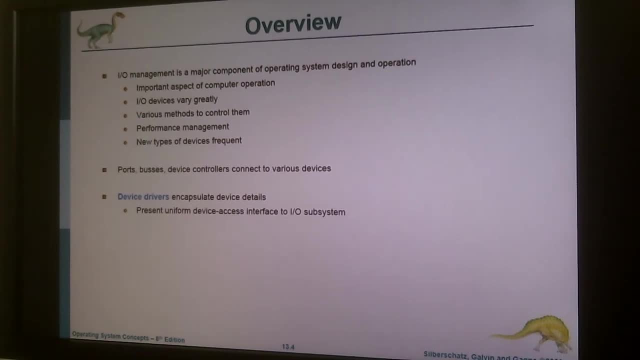 So these are Device drivers works like Communicates with the interface given in the operating system And the operating system will take care of the rest. So what do we have At the end? we have the operating system and the interface and attached device drivers. 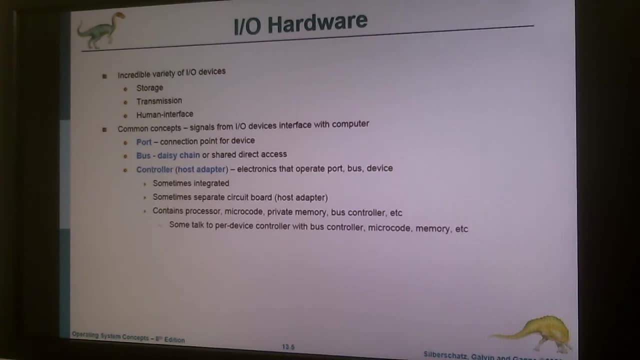 And at the very end of this chain you have the device itself. Okay, We will talk about those device drivers later on. more about that. But what kind of IO hardware, IO devices you see in the market? This is just the general types. 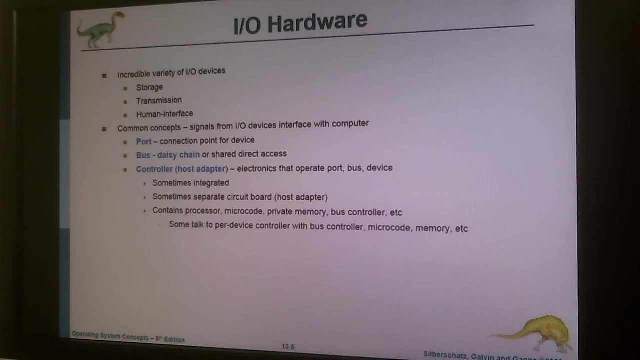 You might have storage devices, transmission devices. What does it mean? What is a transmission device? Something sends and receives something, Some sort of data. For example, your wireless card in your motherboard, your wireless connection, is a transmission device. You can disable, enable that device. 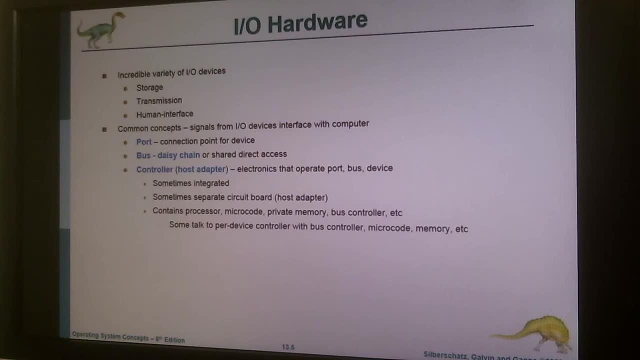 Like Wi-Fi. Yeah, like Wi-Fi, That's right. Yeah, I used the E-download word And also your network card. if you have, you can plug that cable into your computer. What else, What kind of transmission device we can use? 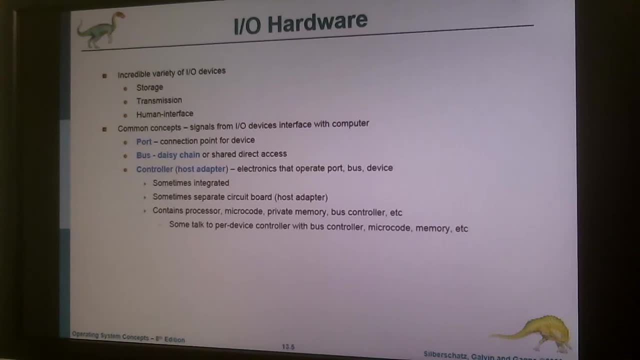 Modems. Well, we don't really have a modem anymore. We don't use them, But still for really, really mission-critical places, in those kind of places, we still use modems as a backup unit In case everything fails. 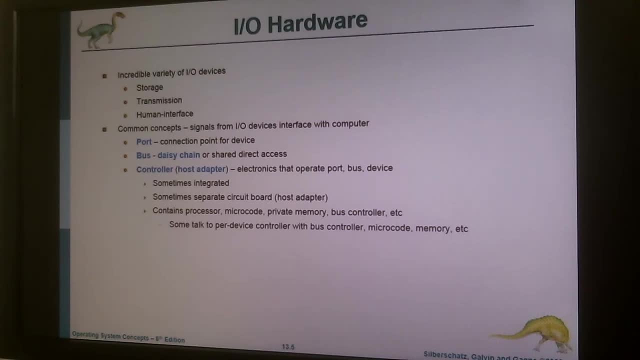 we can still connect to the system through a modem, All right, It is really it's like having an AM radio, just in case. you know, everything fails. you know the whole system. satellites are down, FM channels are down. 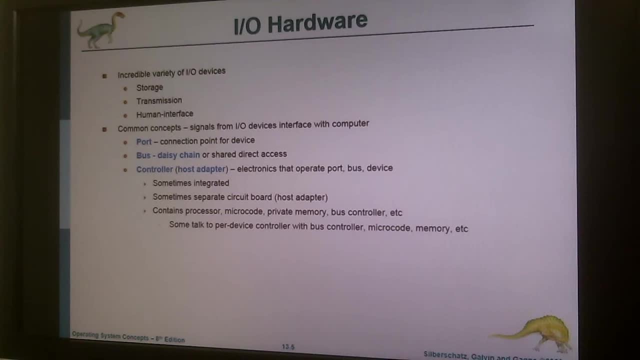 but AM radio works all the time. It works always Because you know, in case of emergency and nuke et cetera, there's always, you know, governmental broadcasts on the AM band, Just like that. 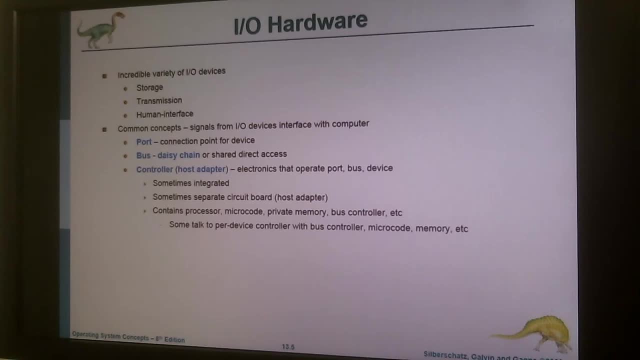 Modems are used, still used, And transmission. transmission devices works like that: They receive and send over data over a wire or wirelessly. What about human interfaces? When I first heard about these human interfaces, I was thinking, like you know. 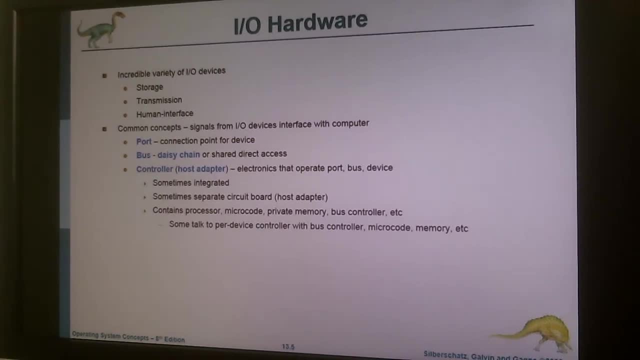 some sort of implant or something. But it's not like that. Human interfaces are devices between the interface, devices between the computer and the people. right, Like what? Like speaker, like microphone, like the display itself. These are human interfaces. 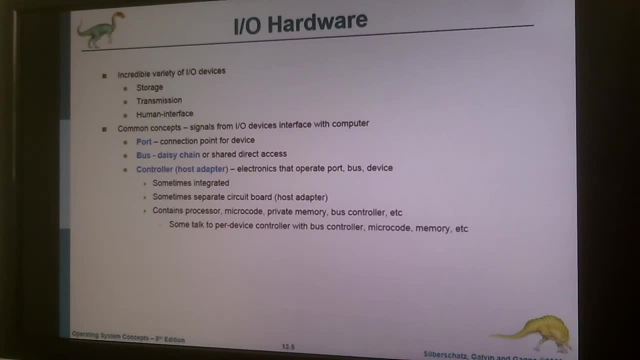 These are the types of wire hardware right And common ways to use to carry signals from an IO device to the computer. you can use a port, a port, like you know, HTTP 80.. That's a port. 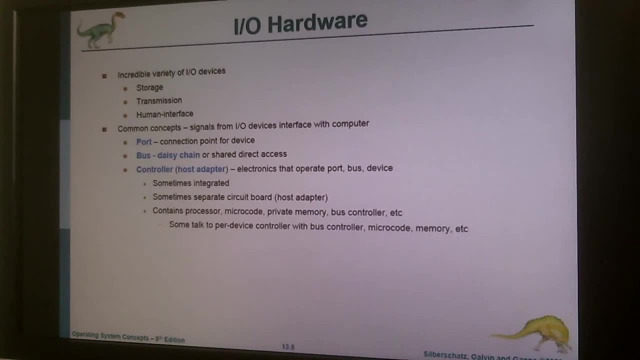 It's a network port. You can use that. Or you can use a serial port. right, That's another type of port. actually, A USB is a port too. You know, there are several types. You can use a bus. 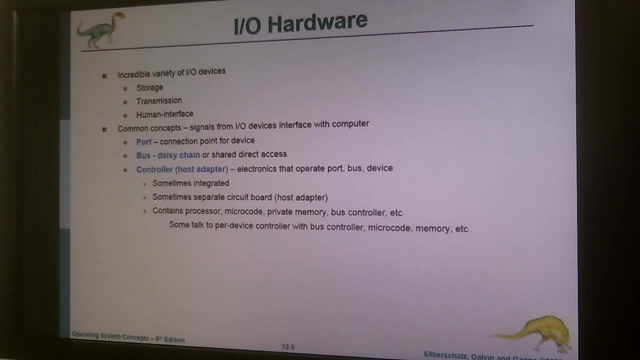 an external bus. This is not like the one inside the computer, An external bus, like how many USB devices you can attach to one single port? One, No, One single port. It's just one single port. How many devices you can attach to that port? 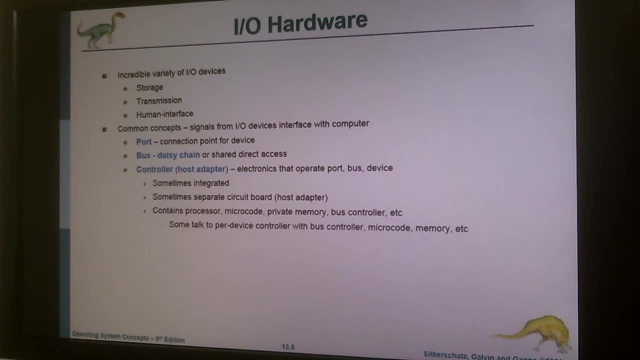 You can use like USB hub. That's right, It's so many. Yeah, you can plug a USB hub and you can actually kind of create a daisy chain. You know, for example, for Cisco routers, Cisco switches, you can daisy chain those stuff. 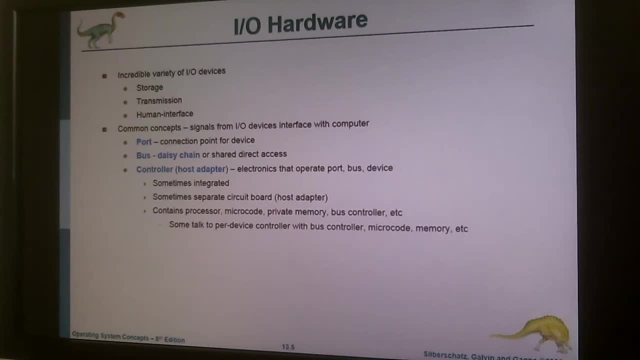 Let's say you have a company in a room, in a floor. Let's say you have 200 people working in the office and you have what is the maximum number of ports on a switch you can have right now? 48?. 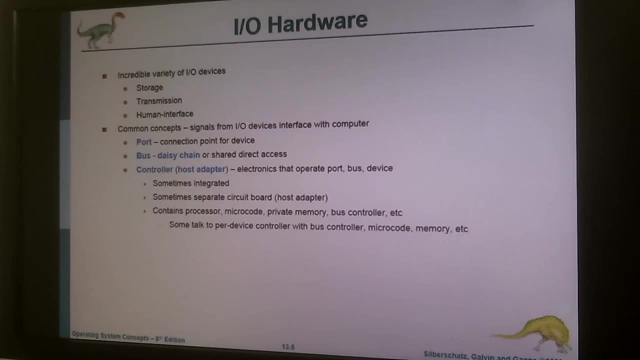 Right. So how many of them you need? Whatever, 200 divided by 48, right, Don't push my CPU cycles. And then you can, just, you know, plug them together to manage them with one terminal. You can do that. 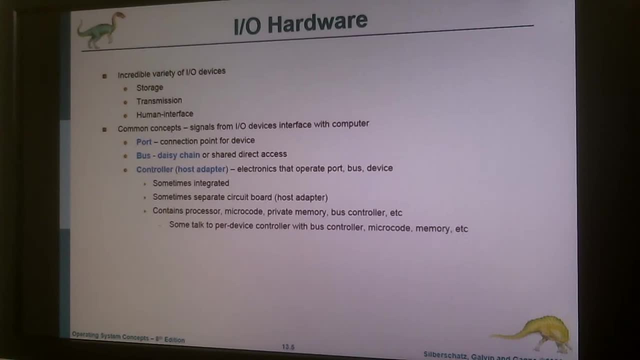 right, Yeah, Okay. And also some ODI devices require their own control card. For example, you remember that hard drive I showed you last week And at the back of the hard drive there was a green PCB. I was saying that this is the controller. 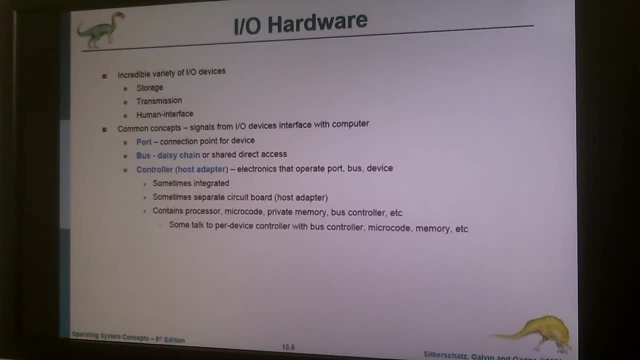 Yeah, that is some sort of electronics, integrated circuits attached on it, which actually controls that real hardware and gives an interface to the device driver on the operating system that you installed. For example, heard about SCSI drives, No, Okay, Heard about RAID controllers. 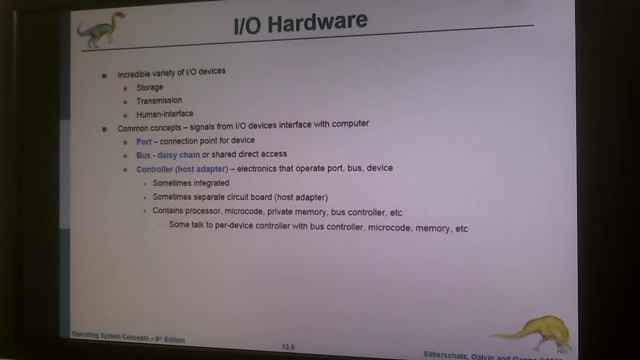 No, Okay, RAID is important somehow, especially for you, for network managers, administrators or system administrators, RAID systems are very, very important, And those RAID systems are used to keep the system up and running all the time, even if there's a hardware failure. 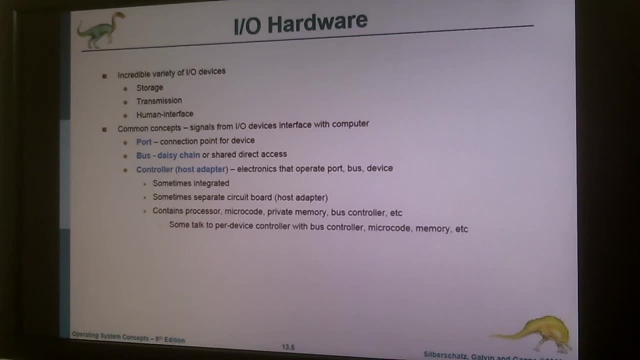 All right, You know you can hot swap those hardware without shutting down the whole system. You know, think about a banking system. If you shut down the system just to replace the hard drive, what happens? The whole banking system will be down for like 10 minutes. 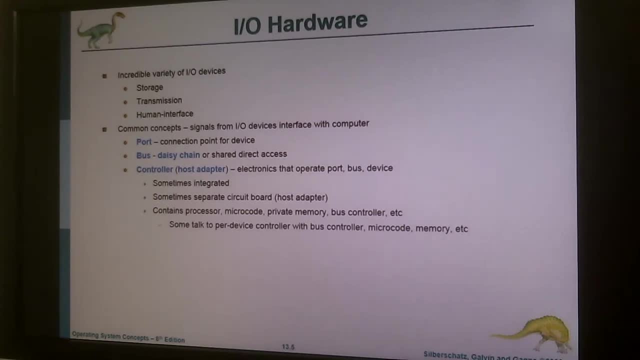 It's a lot of money you're losing there, So it should run. You know, either you can have backup servers or you can have a RAID system that you can just replace that hard drive without shutting down. Anyways, systems require a RAID controller. 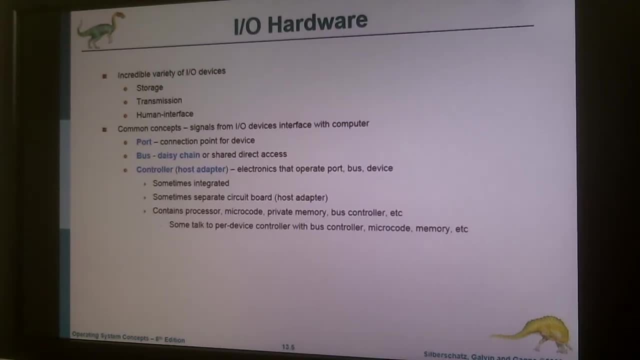 because it's a really, really complicated system. Instead of attaching those hard drives directly to the motherboard, what you do is on the motherboard you have slots right: PCI-E, PCI-X, et cetera. They're kind of slots. 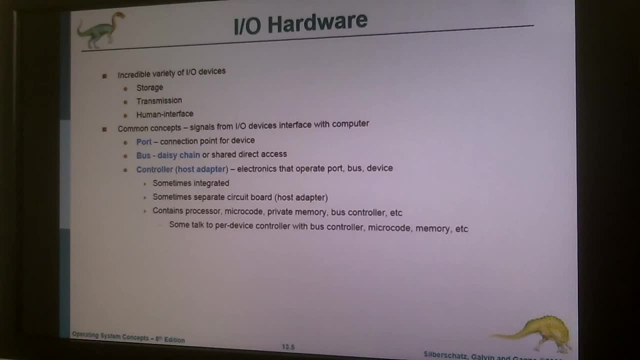 If it's a desktop computer, of course- And you insert that controller onto that slot and install the device drivers, And then you put the hard drives onto that control card. Anyways, that's another way that you can attach your IO devices into your computer. 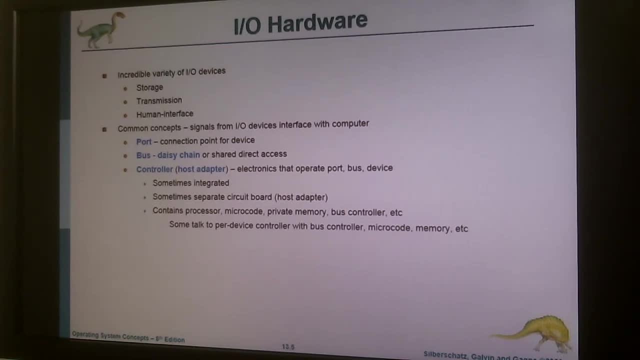 Anybody has a printer at home. Okay, Did you install it yourself? Yes, What kind? Well, yeah, as a CS student, at least I could be. you know, I should be able to do that. What kind of operating system you have? 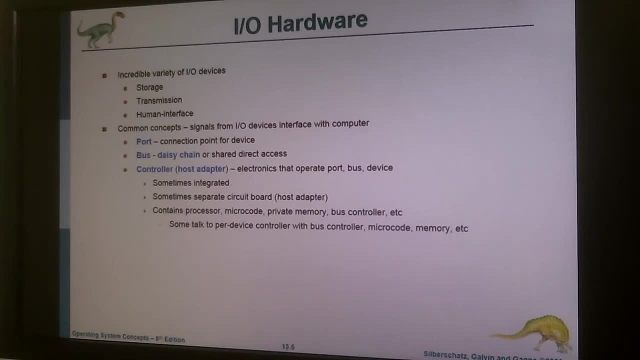 It's all four. It's printer, copier, scanner, faxer. It's a Canon model, I think. Okay, Well, but what's your operating system on the computer? Oh, I can't remember. I think it's compatible with all computers. 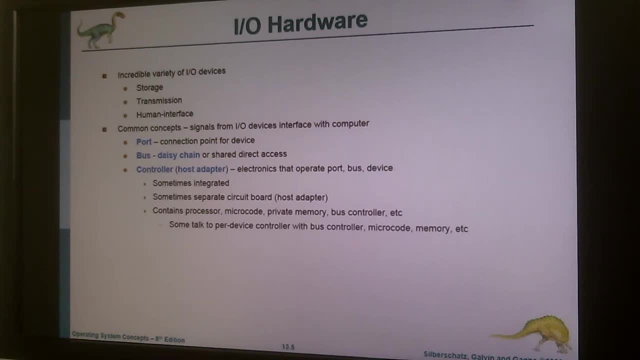 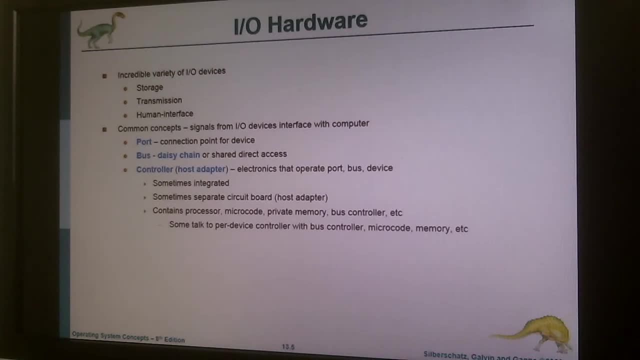 I don't know. I don't know. I mean, is it Windows, is it Linux? Well, the thing is, it actually works with all of them. Oh Well, do you remember the time you were installing that printer? Was there a CD? 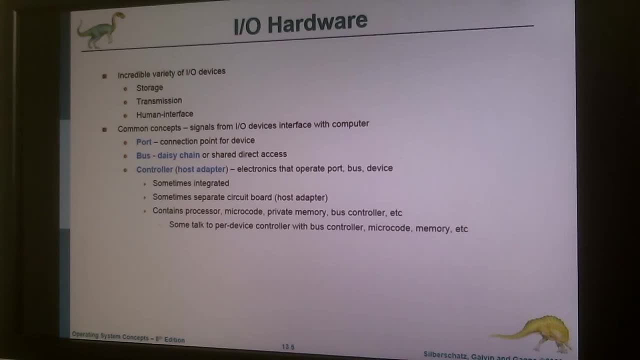 Yes, Do you remember the folders? Was there any Windows, Linux, Mac OS folders? I think it said Linux on it. Well, well, most mostly, you should have all of it right, because you know when you you, when you buy it. okay, what I was trying to say. it's a long story. 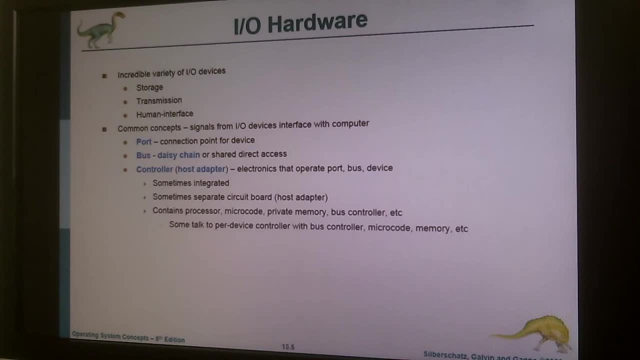 the wise drivers are operating system specific. that's what I was trying to say when you buy a printer, so we have been installing our system, right, okay? one more question then: do you have to install all the drivers from the printer all the time, or does it work? 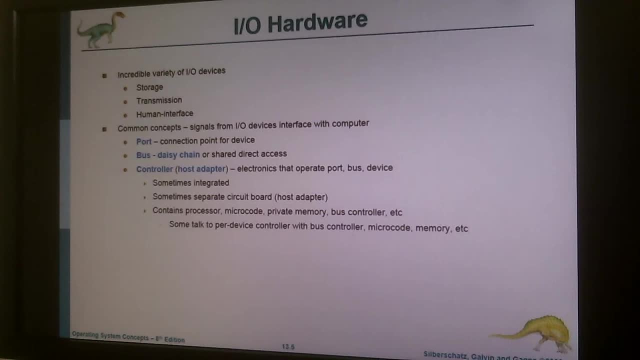 sometimes without any drivers involved. yeah, you have to install. you say: what about default Windows drivers? what about that? yeah, you know, most of the devices are built in. right, that's right, okay, one more question: if you install driver, your printer will work. so why do you need? 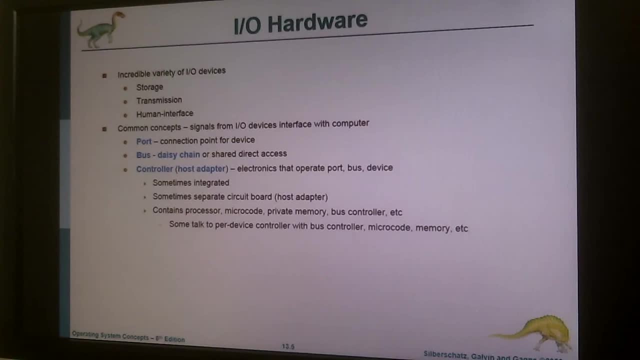 an additional software like printer controller or whatever. it shows you the ink levels and other stuff. why do you need that software? any others ideas In marvel that software, ingredients, whatnot? What kind of application that you're installing for printer management? you know comes with the manufacturer. 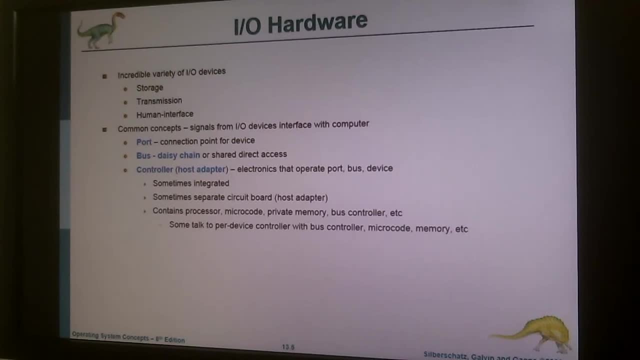 What kind of application is that? Running your own business? I suppose I don't know. All right, Is it a user application or a kernel application? User application: It's a user application to help you to manage your printer and, you know, to see to. actually, you know most of the printers right now. they're inkjet or laserjet, right? 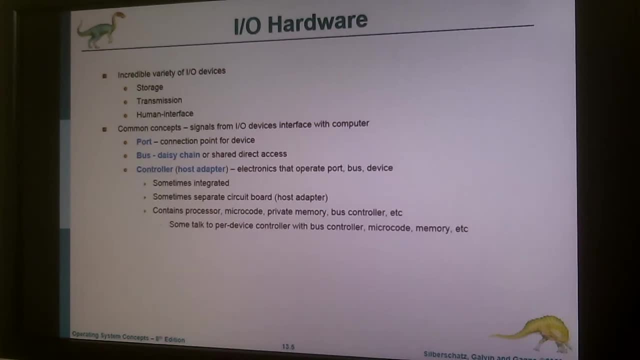 Is there any other types? You know, I don't really know. I mean I know some sort of. I have fixed a printer years ago which uses little colored cubes. It just melts that. It's not inkjet. It melts that cube. 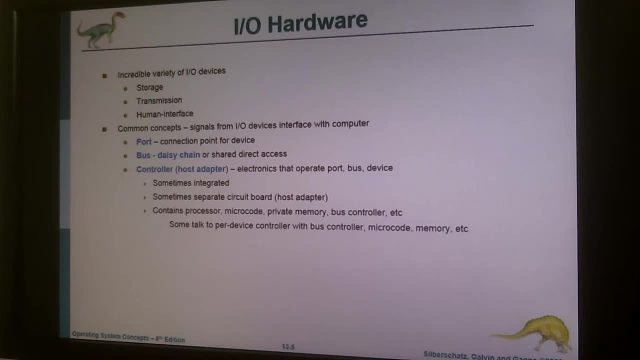 Okay, Literally with heat, and then prints it on the paper, which was super high resolution. It has a, you know, high resolution output used by graphic designers. It's a huge and super expensive printer. You just buy the cubes of colors. you know: red, green and blue. 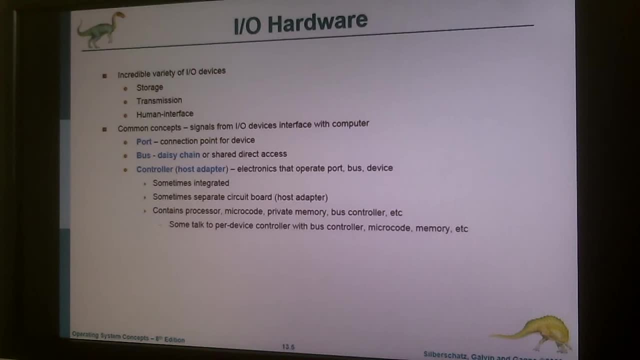 That's crazy. That was the first time I saw something like that. I mean, whoa, What is that thing? As I said, it literally melts that, And with the heat. Anyways, that software you're installing from the manufacturer is not a driver, but it just helps you to maintain your printer. 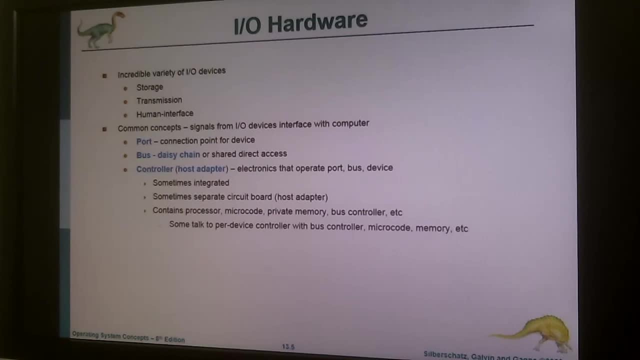 You know, you can see the print cues. You can, you know, manage the jobs in the print queue. It's for feedback. right, For the feedback too, It can actually automatically look to the manufacturer's server and tell you: hey, there's a new driver. 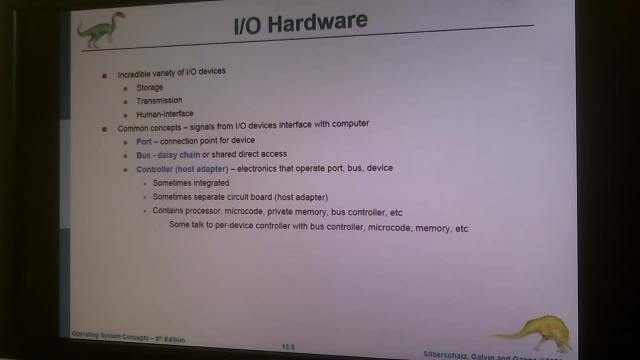 You want to install it. Hey, there's a new application. you know the new version, new update or whatever. What do you want to do with that? And also, some of them actually enables you, enables actually your printer, that you can actually print to your printer at home from the Internet. 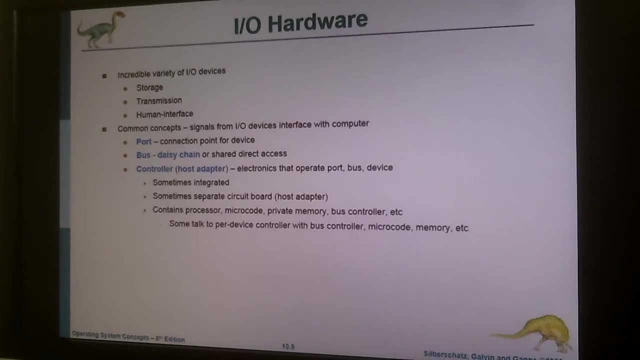 So you're a student here and you're trying to print out something You don't want to forget about it, And then you just send that job to the printer at your home or office or whatever. over the Internet You can do that. 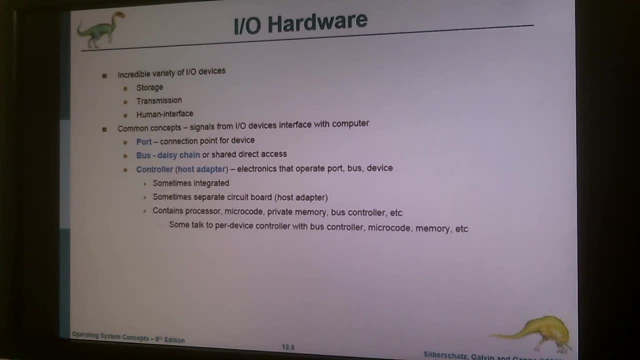 It can print that thing you know, remotely. Those kind of applications helps you to do fancy stuff like that, all right, But they're not drivers And sometimes you will see that, you know, while you're installing the application they will ask you: do you want to install the software and the driver, or do you want to install just the driver itself? 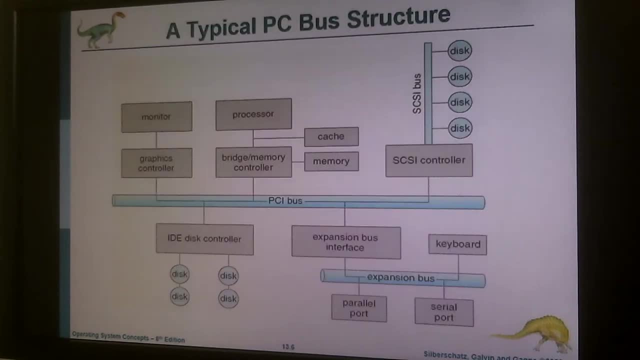 All right, You know you will see that kind of custom installation stuff And this is a typical PC bus structure. on the motherboard inside your PC, inside your computer, As you see, there's this PCI bus and you have all these controllers for every device. 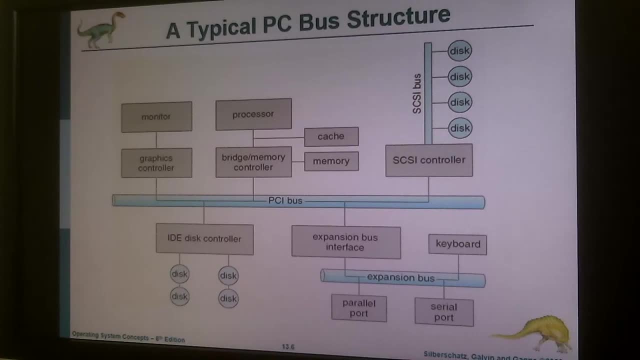 All right. so if you imagine that you have a physical device like printer or whatever, and then you have a controller card or device And this is a typical PC bus structure on the motherboard inside your PC. And this is a typical PC bus structure on the motherboard inside your PC. 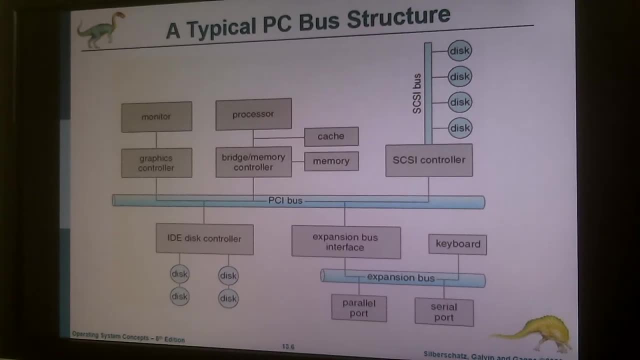 And it's built on the motherboard itself, And then you have the device driver And finally you have the operating system. So this chain altogether makes the iOS device work properly. right, That's the way it works. For example, here you have the monitor, the screen. 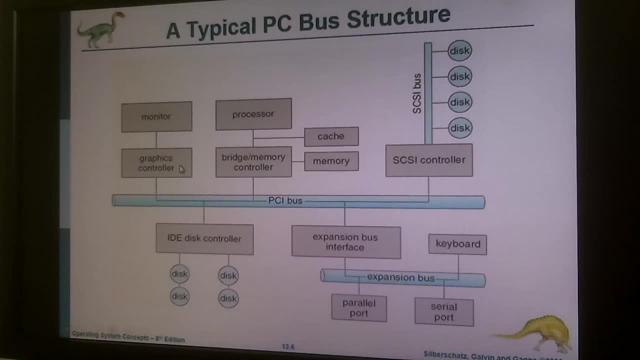 You need a graphics controller, VGA or SVGA in the old days. Now we have HDMI. other stuff. for the disc you need a disc controller. actually, this is every disc has its own controller, as I showed you attached to the metal, the aluminium container of it, but this one is look like a rate controller you attach. 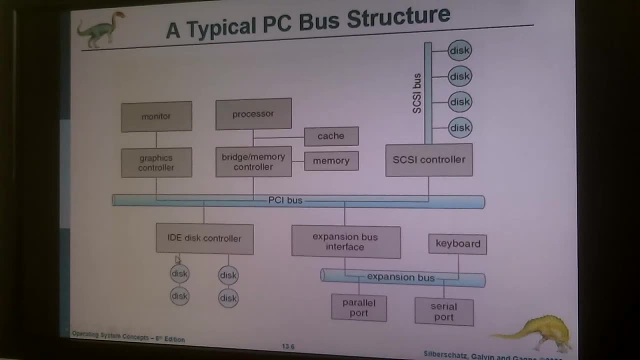 multiple IDE, which is an old-style, old-fashioned interface for a disk drive, so that you can have a rate system here. and there is also what is that? SCSI controller? this is also a. this is super fast actually, if you compare with IDE or SATA. it is fast, it is expensive and it has its own controller, you know. 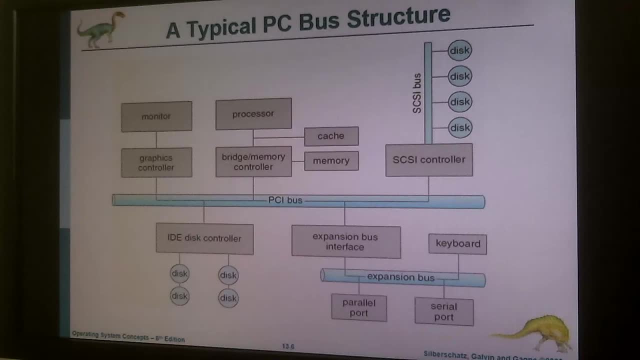 you can use it for a lot of things. and you can use it for a lot of things. but extend, easy, chain multiple SCSI drives with one controller. it was kind of really a choice of system administrators back in the days, but right now I don't think anybody uses it anymore. there are extent extended versions of. 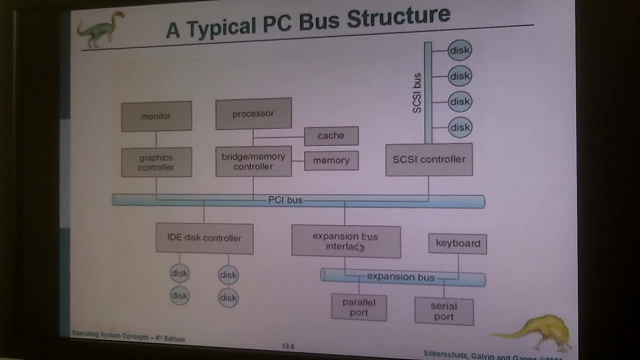 it in the market right now and this one. here on the right double bottom hand you had the slow of devices. these are relatively fast stuff but these are slow devices like the keyboard, like a mouse or parallel port of serial port. question for you, network admin: how do you connect to a Cisco router? how do you log in to a 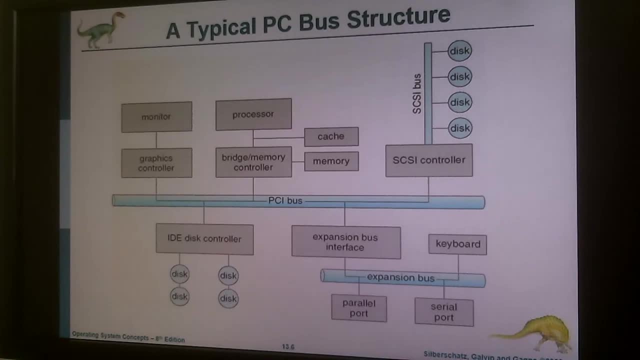 Cisco driver if you don't have Ethernet. what is that console port is actually how many pins you have on that console port. no, that's actually report. we're talking about the console port. oh, maybe you're right. maybe the latest ones are not using RS 232 anymore, they use RJ 45. 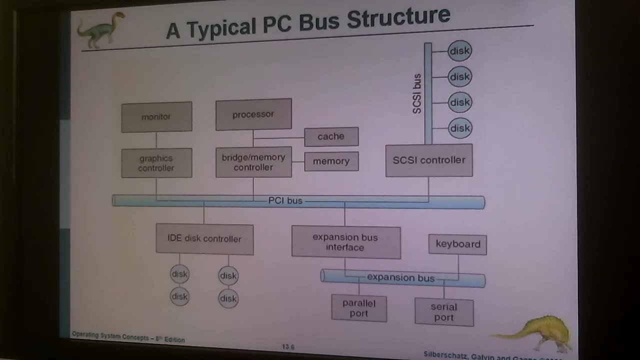 right. you might be right, I'm not. I'm kind of. you might be right, I'm not. I'm kind of. you know behind the tech on Cisco's, but in general you have a serial port on a Cisco device. you know when you buy it from the manufacturer for the first time. 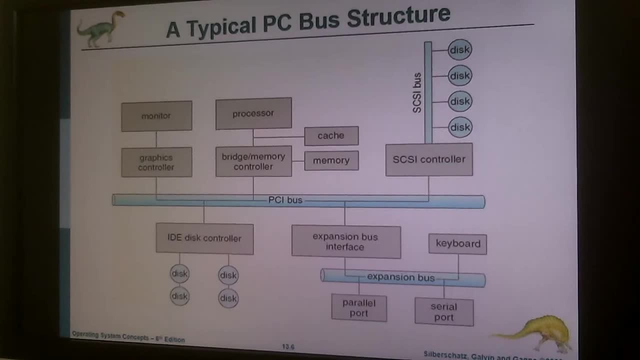 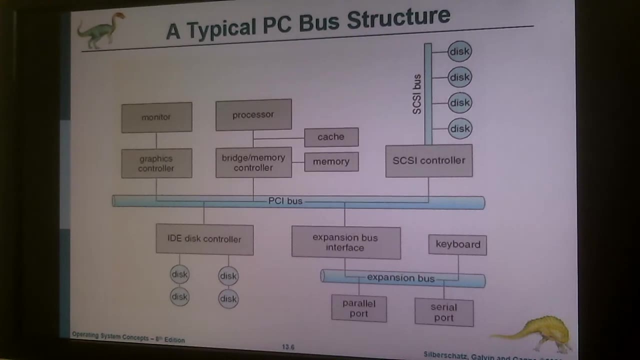 it will have a default IP number. you can connect with the internet, but the best way to do that connecting to it with a serial, through a serial port. when you use that serial port you can configure everything. you can backup the configuration and upload a new configuration. let's say you have. 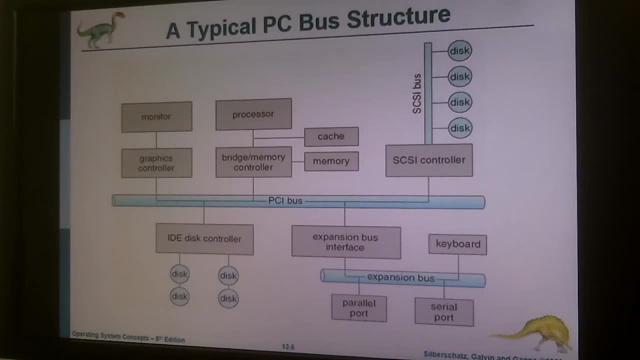 similar models, many routers. or let's say you're trying to implement a configuration, a fixed configuration, to many devices. what would you do? you will just connect through the serial port, just upload that configuration file to each of the routers and then, of course, you have to change their IP addresses because they 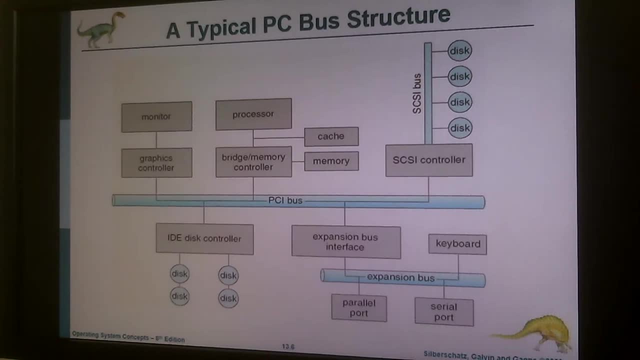 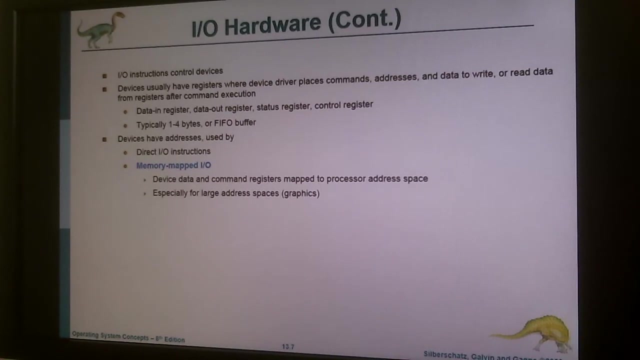 cannot be the same right. all right anyways, there are multiple ways to do those kind of what is that? benched batch of jobs, unattended installations? you can do many. you know you can use many tools in the market, open source to including open source ones, all right. 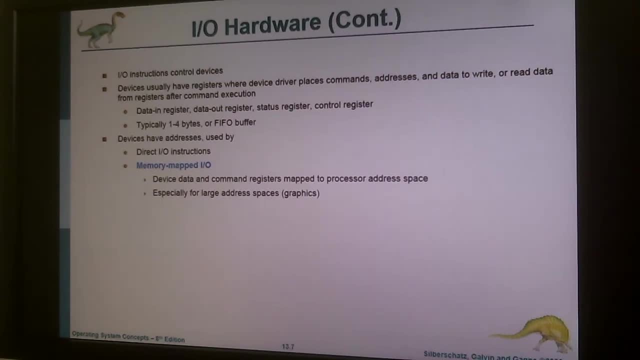 what else we're gonna talk about today. all right, you can. you, after installing your device drivers. now you're you're going to be able to center the data to your device and applications can use your device. for example, Microsoft Word can print to your printer without using any other. 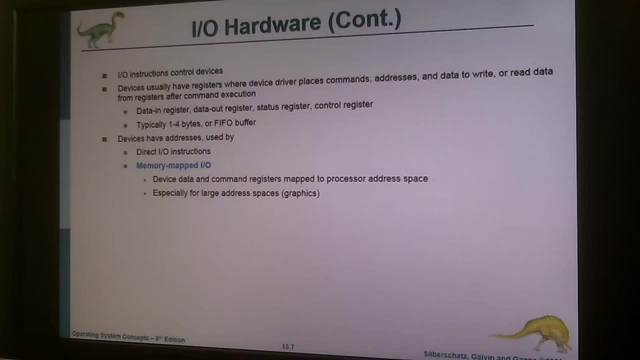 additional stuff because the device driver will handle everything all right. when you install the device driver, you will see it in the hardware list and it will show up as a printer device in the printer list and when you're printing from the word or any other application it's gonna be usable for you, that is. 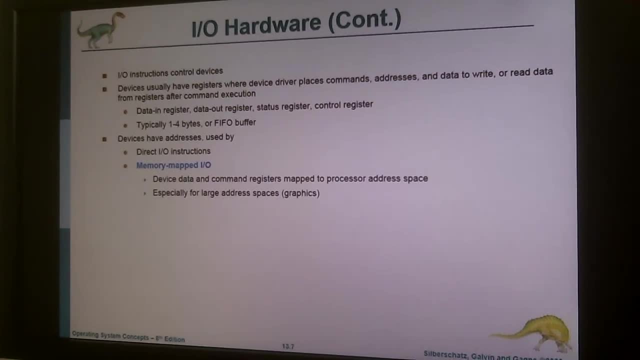 through the IO bus. but there's another way to talk to the IO device. you know if you're moving- for example, if you talk about, think about the hard drive- you're moving a large amount of data between the device and operating system, right? sometimes you're just copying a big file like three gigabytes or more. 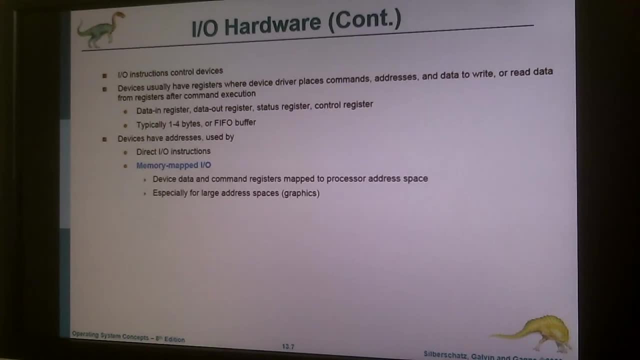 right, sometimes you're just copying a big file, like three gigabytes or more, from the device to the memory, the physical memory, so that you can work on it. right, like you know, you're trying to edit a photo, a big photo file, in Photoshop. that is possible, right? it's most likely the case, actually. so if you 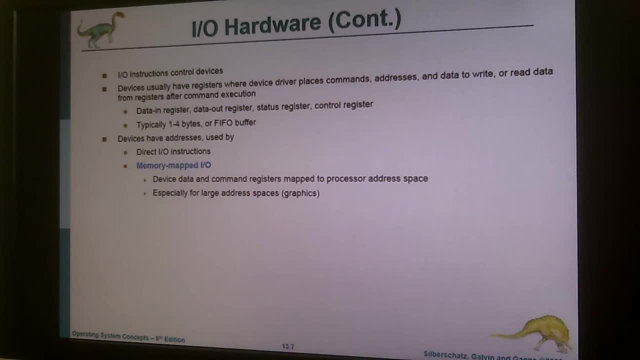 use a regular device driver approach. in that case you're gonna fail, because only device driver, using only the device driver itself will not, will make the CPU very, very busy because you know it has to talk to the operating system, it has to talk to the device driver by 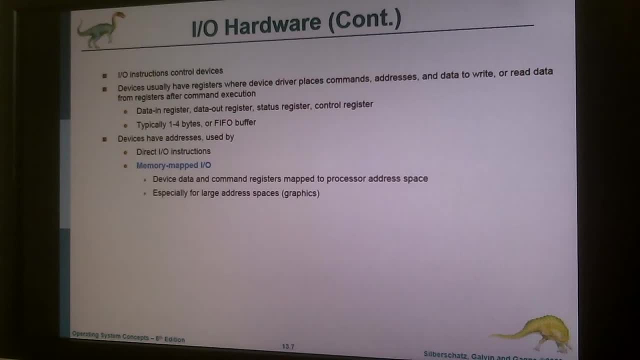 the way is a bind, is an application? all right, it's like a bunch of system calls but talks to the kernel directly. it's a program, it's an application. but it's a small application which enables you the communication between the operating system and the device. right, but in for large data movement. 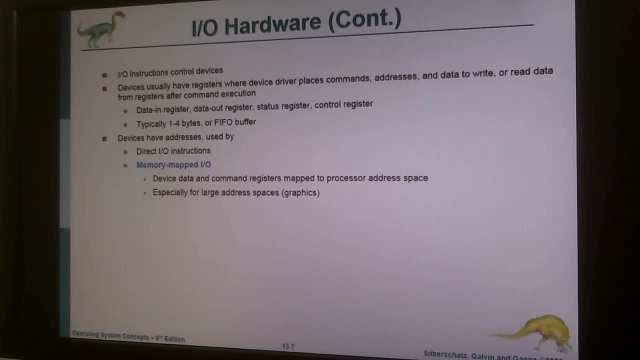 and the device driver itself, using its memory only or physical memory, the RAM memory on the system, will make the CPU very slow because of the- you know, lots of, lots of communications, lots of processes, memory dependent. instead, there's another way to do that. you know. actually, again, you're using the device drive. 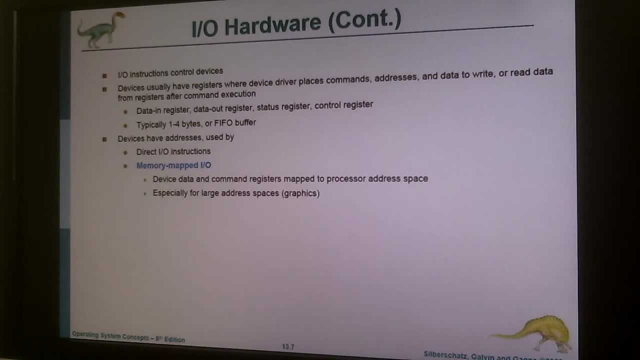 driver. but this time, instead of using the memory on the system you're using, you're using some internal memories on the device, plus something called direct memory access, which actually makes the CPUs job easy because it doesn't have to manage that memory through the CPU and the driver. it just puts data from the 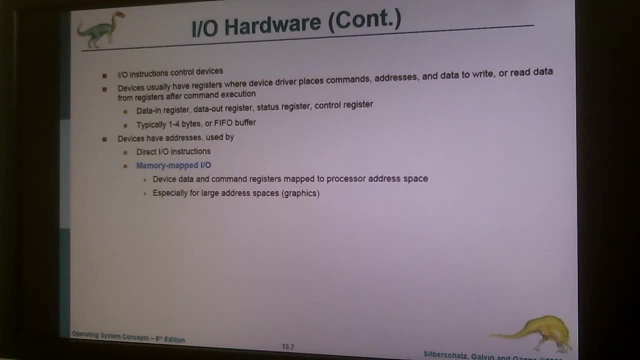 device to the physical memory and the device driver, in this case, doesn't go to the CPU and ask: you know how can I connect to the Aie device? let's get some data from from it? instead of doing that, it just looks at that specific location you know, between the device and operating system there is. 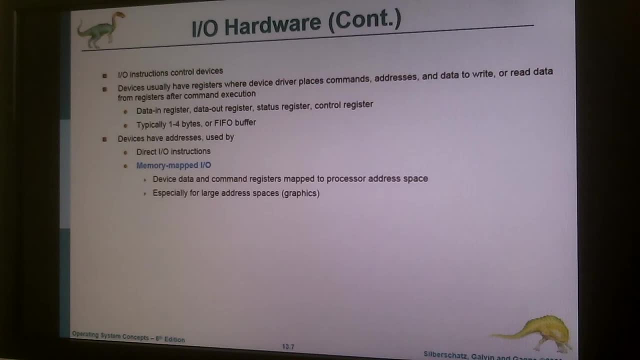 this memory space. it doesn't look or ask to the CPU to manage that space. it will just take the address as a parameter and look at that space. when you're moving a large amount of data, specifically, it will help the operating system reduce a lot the CPU cycles and the load that is actually. 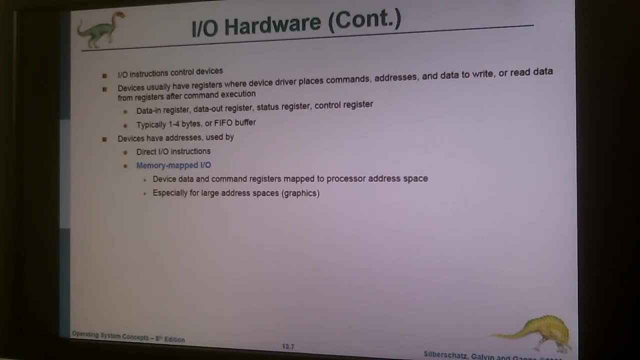 called DMA, direct memory access in most of the motherboards. latest computers have a special DMA controller microcontroller installed on the motherboard. those memory management parts, or the memory map mapped memory, will be a job for this little micro microcontroller on the board. today it is called the DMA controller. okay, it's not your CPU anymore. CPU will be free. 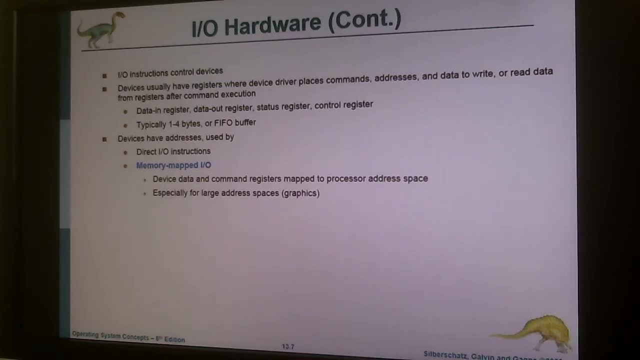 instead, this microcontroller will do the job okay. so DMA actually helps a lot to speed up the system. but there's one problem with that, what it could be. you're accessing to a system memory without asking the CPU or, in many some cases, without even asking the operating system, because you 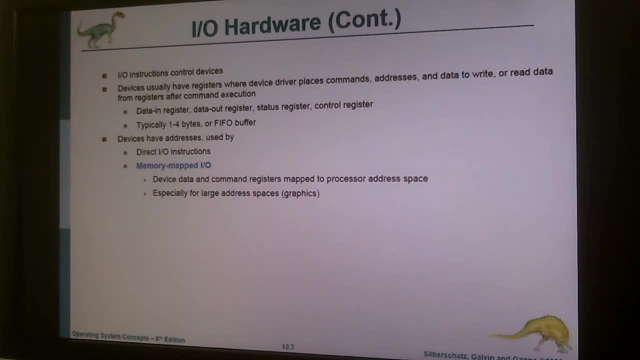 know you don't have to use the system code of the operating system with the DMA. you're not actually buttering this operating system in the CPU with those calls and you're just handling the with external devices like the external microcontrollers and the device drivers you wrote. you're actually bypassing the CPU. that means you're also bypassing the. 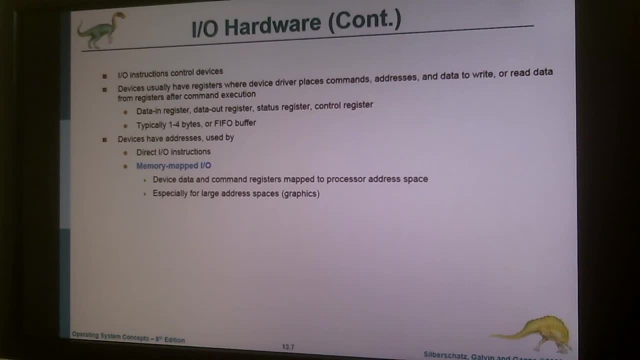 system security. right, that is actually a problem, a protection, a security problem for the whole system. because you're saying, for example, your device driver will say: you know, I'm going to use this 200 to 300 memory area for my DMA access. that's what you're saying, but in your code it's a malicious code. you wrote it. 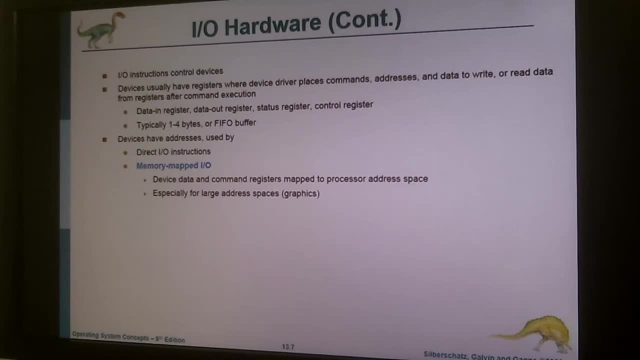 instead of 200 to 300, you're using 0 to 100, which is a system space, and you're crashing the system, right? yeah, that's a wires. let's say so that DMA access given to DMA. that's a virus. let's say so that DMA access given to DMA access given to. 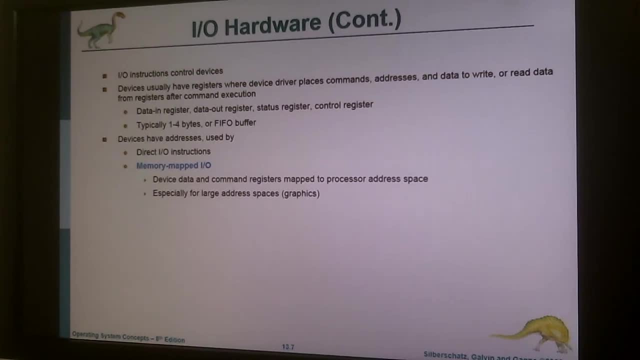 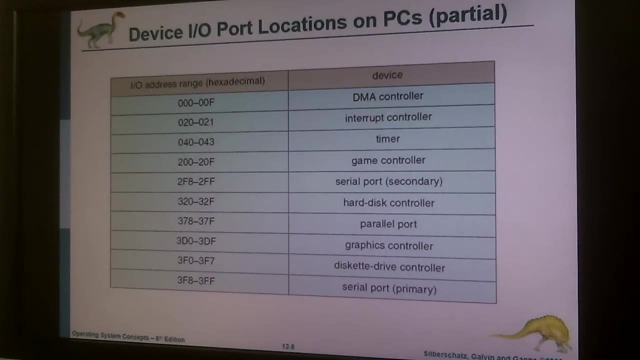 that device driver in this case is not helpful. It's very harmful for the operating system and for the whole thing, for the whole environment. Some of the very well-known device DMA ports. I'm sorry the address ranges, not the DMA only. I'm sorry it's the I-address range. 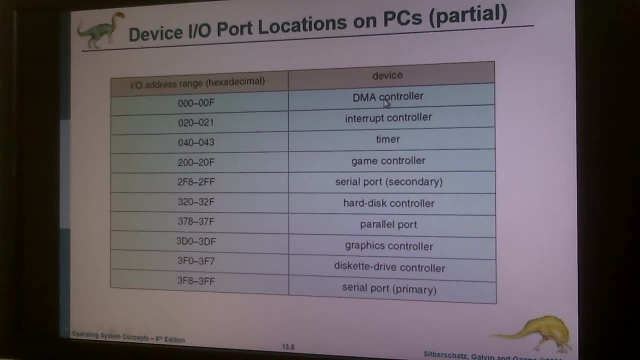 The DMA controller is an additional microchip. it's a microcontroller on the motherboards and it uses the I-address range 0 to 0F. this is hexadecimal And this is just an example. these numbers are not absolute. these numbers are not even specific to any operating system. 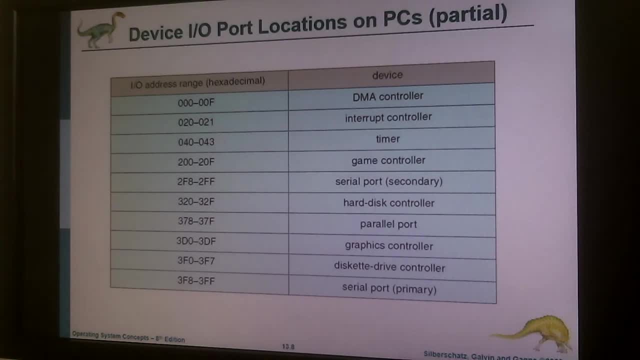 like Unix or Windows, but this is like in general. For example, the intra-app controller uses this address space. By the way, when I say I-address space or I-address range, what kind of numbers are these here? What am I actually talking about here When I say address? what I really mean? 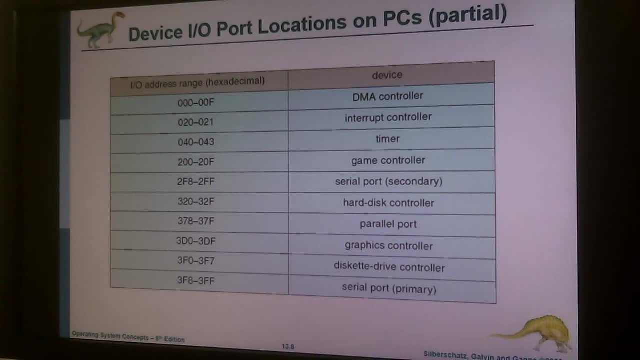 is address on the memory- all right Address. the only thing that might have an address is your memory stuff, all right. So these are on the physical memory. The timer information game controller: all right, game controller means joystick, Serial. 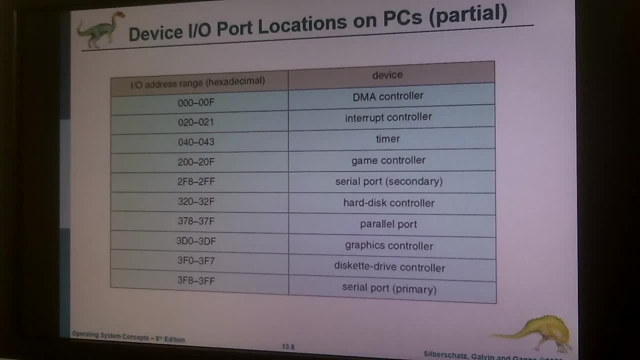 port secondary hard disk controller. parallel port graphics controller. diskette drive. Okay, there's no diskette drive anymore. You can use this area for something else. okay, So serial port, primary one. In the old days, when you buy a motherboard, it would come with two serial ports and one. 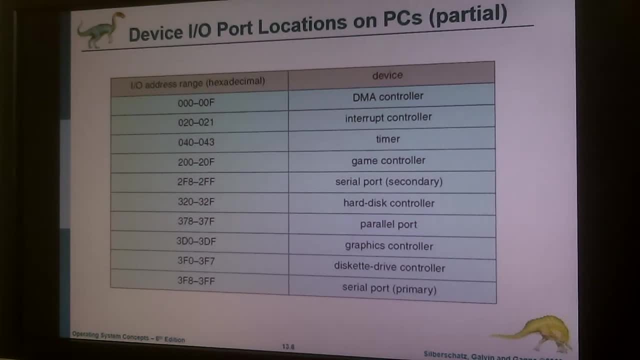 parallel port. Now, there's no parallel or serial ports on any motherboards on your laptop. but what you can do, if you really need a serial port for your old Cisco router, for example, what you can use is a USB to RS-232 or serial converter. It's a piece of cable with some electronics. 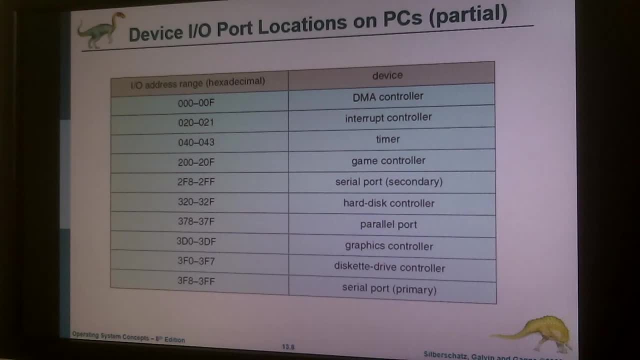 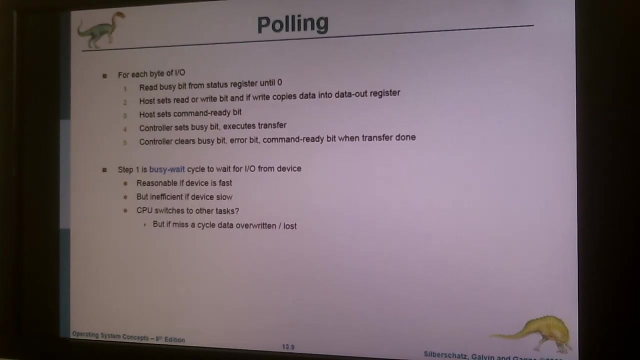 is installed in it. You could just install a driver if you have done it before For that cable. because it has electronics on it, you have to install a driver too. Pulling- Do you remember those CPU scheduling queues? If there is an IO request, what we should do, you know, since the IO devices are always. 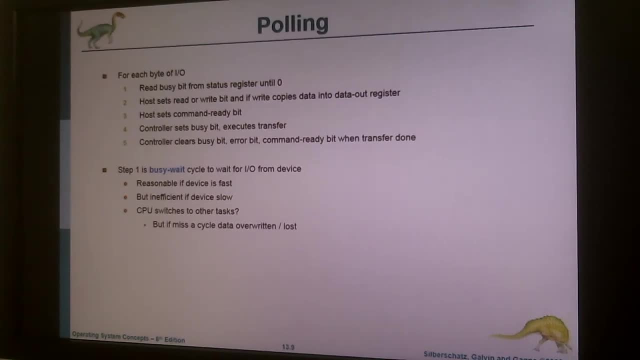 slower than CPU and memory. you'll have to wait for it. Yeah, And what do you do with your process? You move your PCB process control block to where To HQ, right, And it just sits there until you receive information from the IO saying that okay, I got the data. 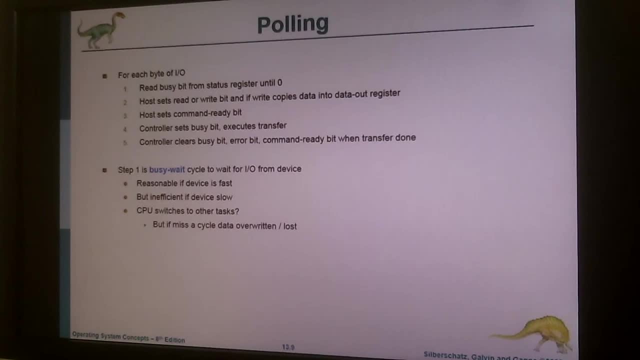 I'm ready, Hello. And then it says, okay, this process has to stop or reload it and then execute it completely, because I had the data from the IO device, from the hard drive or whatever. Yeah, And then you can just execute and finish it up. 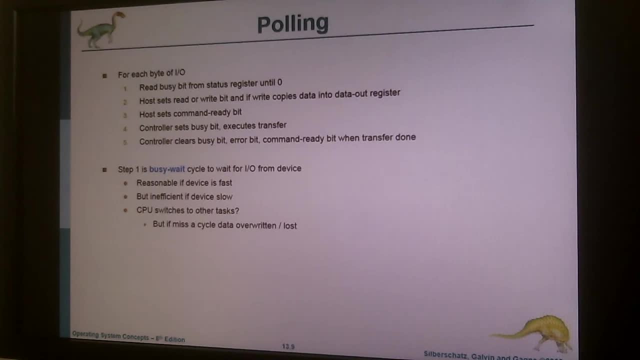 But you have to wait. That is why we have the wait queue, right? Don't forget about that one. While I'm waiting as a CPU put that PCB onto the waiting queue, what do I do next? Let's say. let's say I'm downloading a movie. oh, that's something illegal from. 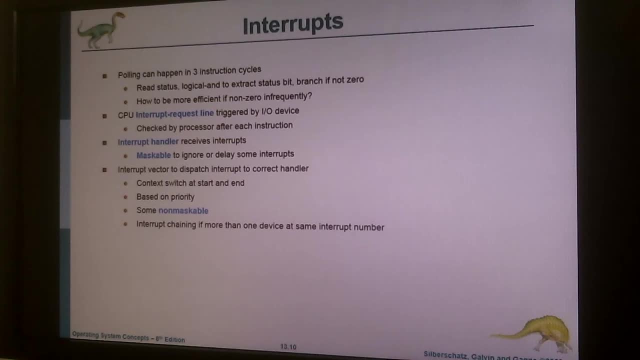 somewhere, and that application that I use to download the movie is called, let's say, BitTorrent, BitTorrent, And that is a busy, busy process at the moment, right, Because it's downloading stuff and it's waiting a lot for the IO, right. 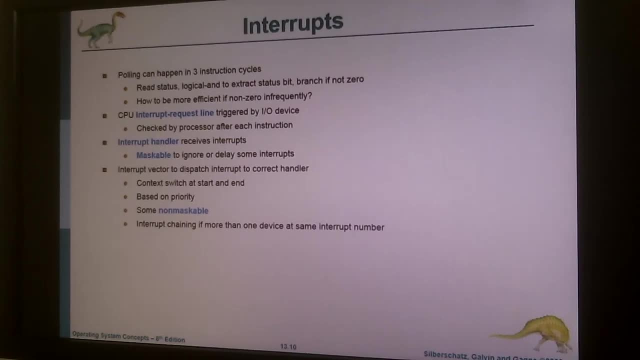 What can I do with my CPU time in the meantime? I just put that PCB into the waiting queue Right And save the state of the PCB and then do something else. whatever you want to do, You can type your diary on your Word- you know file- or you can open up and read some. 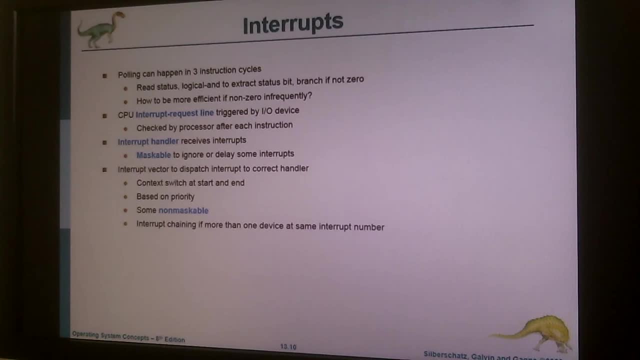 stuff, a PDF file, et cetera, Or just leave the computer all alone. it will just take care of the operating system processes in the meantime. Every CPU has an interrupt request line and those IO, DMA requests, memory map requests. 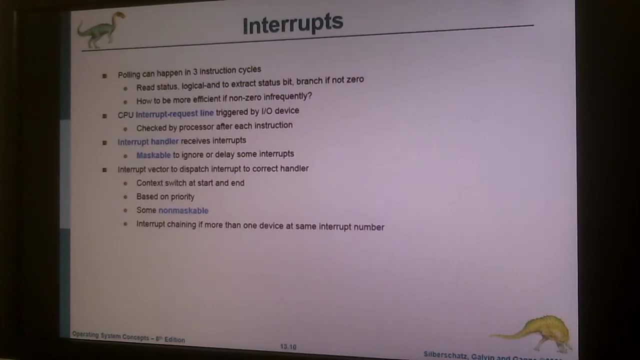 and all sort of IO operations are actually told or signaled to the CPU through those interrupt lines. For example, you're trying to read a file from a CD, right, And that CD tries and tries. it's not really clean. It tries, tries, tries. 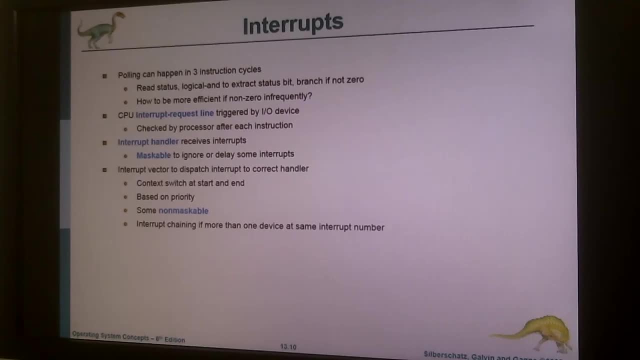 In the meantime, your CPU thinks that, oh, this IO is keeping me busy very long, Let me put this in the waiting queue. and then puts in the waiting queue till when? When are you going to know that the file you're trying to read from the CD it is actually. 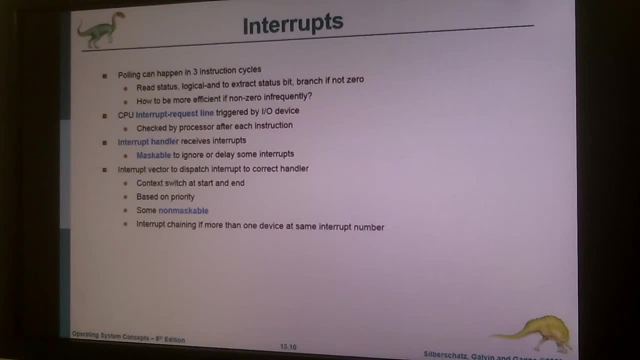 read: How do you know that? How can you know it? There's no process running, because you just save it. You just save that process, the PCB, into a memory space, and put it into a queue. throw it into a queue.